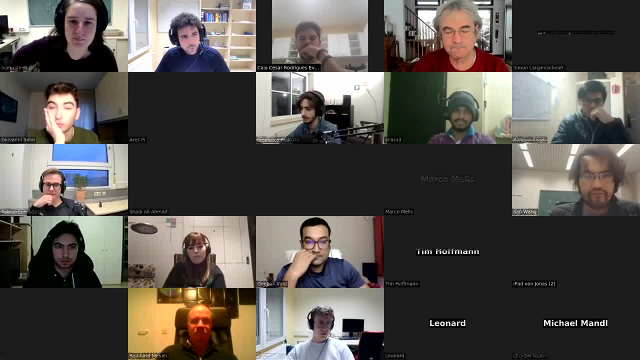 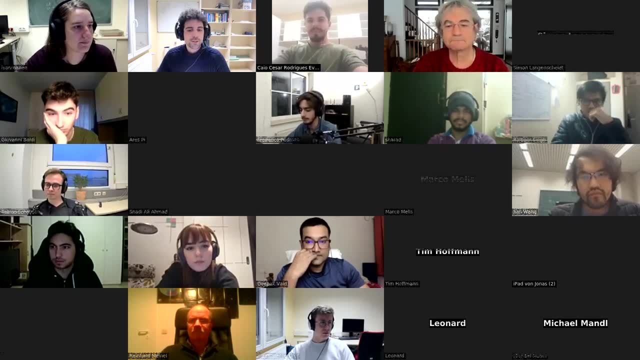 Perfect. Let me also mention everyone that we do have a form for anonymous questions, in case you don't feel like doing it explicitly. So if you feel more comfortable, that's also a possibility, And the link for that will be posted in the chat. 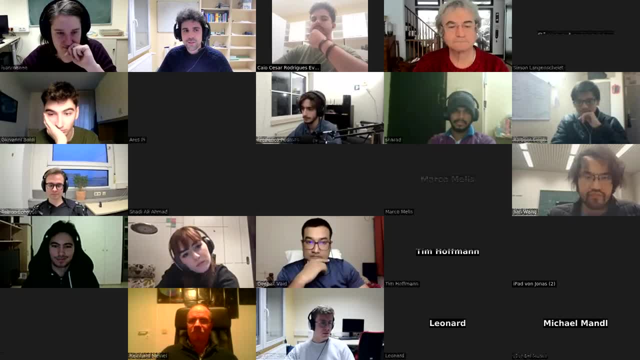 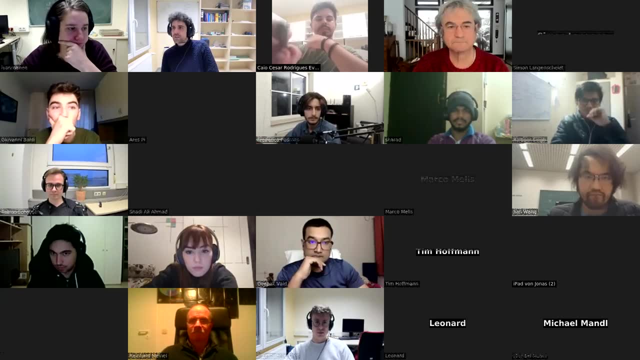 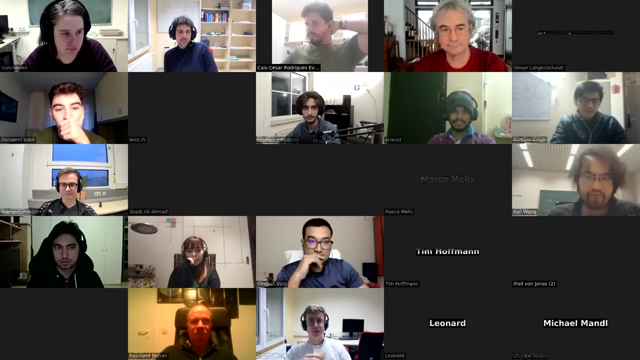 and has already been posted in the chat, but it will be posted in the chat again more often. So, yeah, Are we recording? Yeah, OK, good, Then let me start. Then I have to fulfill the protocol obligation of introducing Carlo, which of course, is a very difficult thing to do. 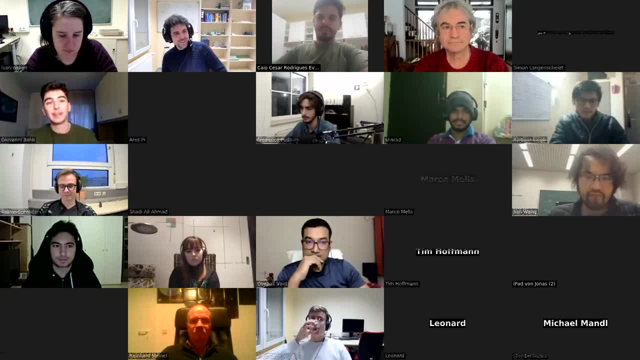 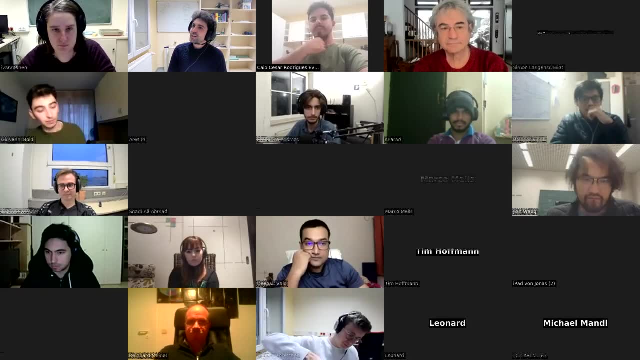 In some sense he needs no introduction, but I will still do my job and try to keep this at the minimum. So Carlo's alma mater, in some sense at least, where he did his PhD, was University of Padua in 1986.. He's currently a professor in the Western University in Ontario, possibly still in Marseille as well. 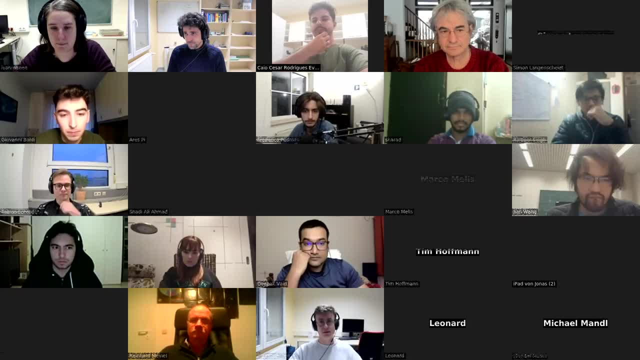 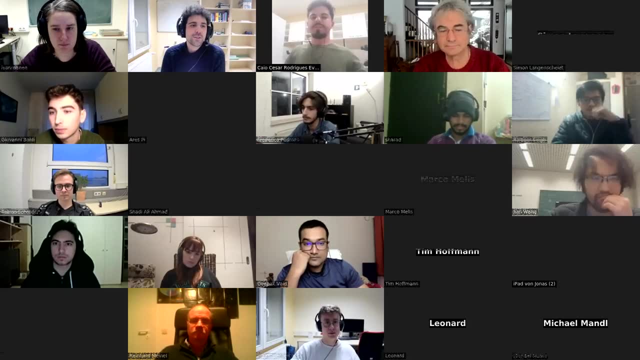 and also holds a chair- a visiting chair- in the Perimeter Institute. Of course, Carlo is an accomplished researcher in theoretical physics, And I will, of course, come back to this point soon, But I'd also like to touch on things that go beyond this. 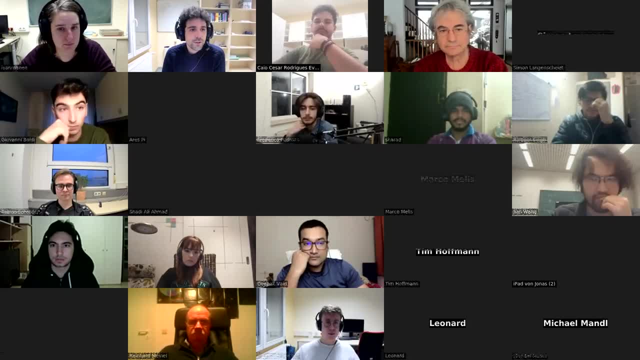 Some of Carlo's interests also touch on, of course, history of physics And philosophy of physics, epistemology- I remember Carlo had the more or less recent paper on Aristotelian physics. And Carlo is, of course, an important contributor to scientific outreach. 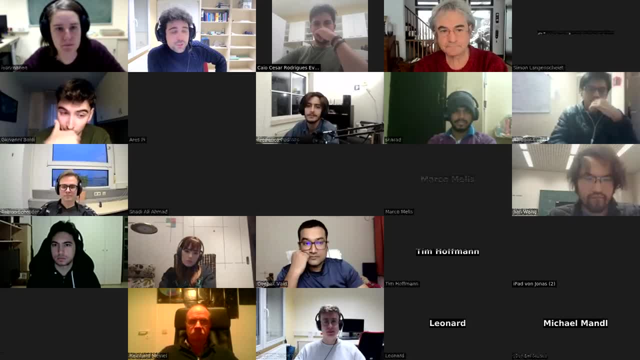 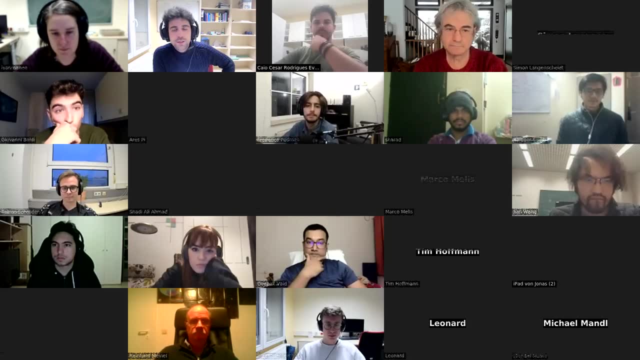 He has a number of of popular science group books, which is, of course, an important effort from the physics community to to reach people that might have interest in physics But they are not physicists themselves. The most recent book he's he's Elgoland on the topic of quantum mechanics. 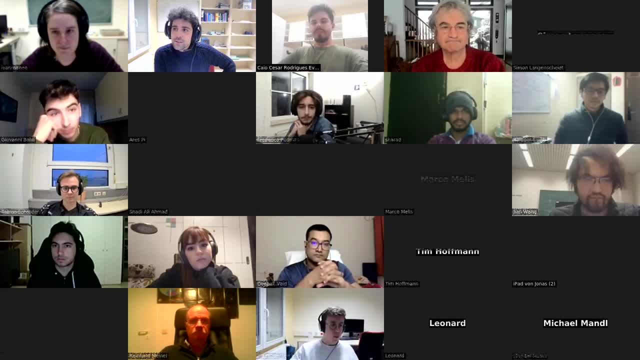 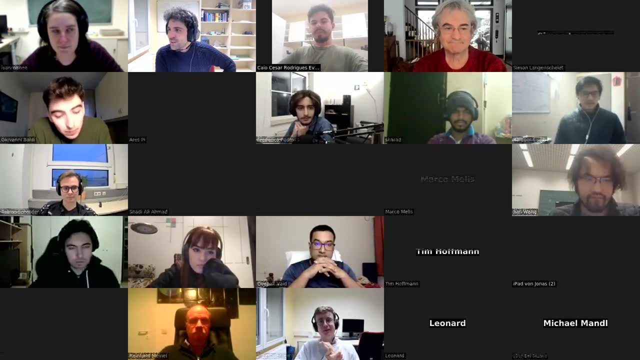 And it's many interpretations. Finally, before the physics part, I cannot resist, but to touch on a point. The fact that I learned about today is that Carlo recently actually co-released a song in November last year with an Italian band, Prima Donna. 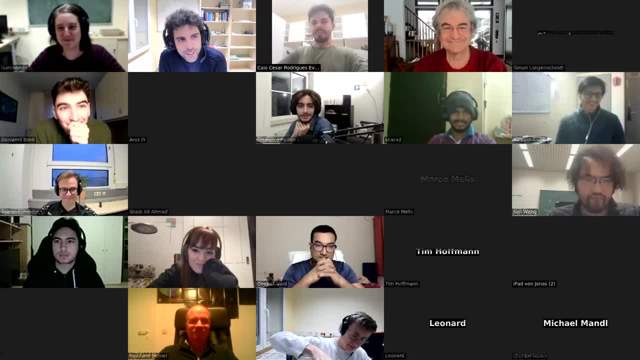 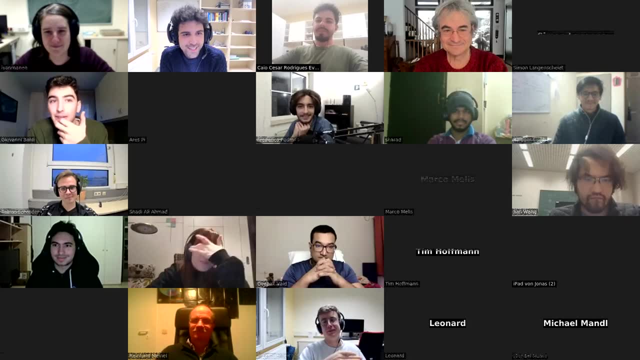 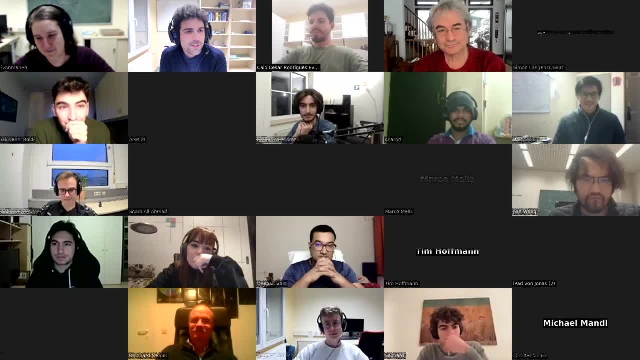 We're here because of him. We're here because Carlo is one of the founders ofenin the great Together. we- and I believe this is precisely what we'll hear about today. So please go ahead and thank you very much. Thank you, Well, this was very nice. Thank you. 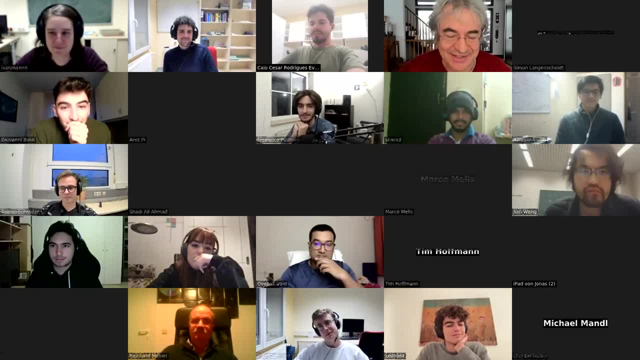 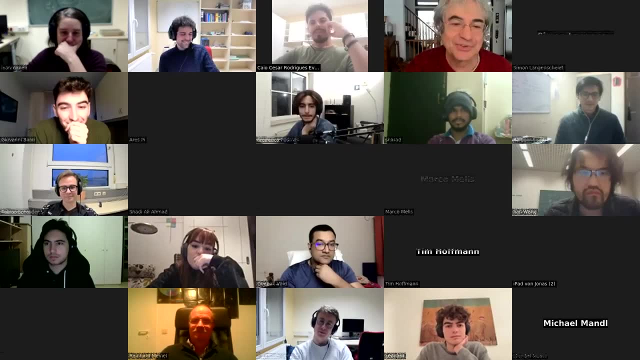 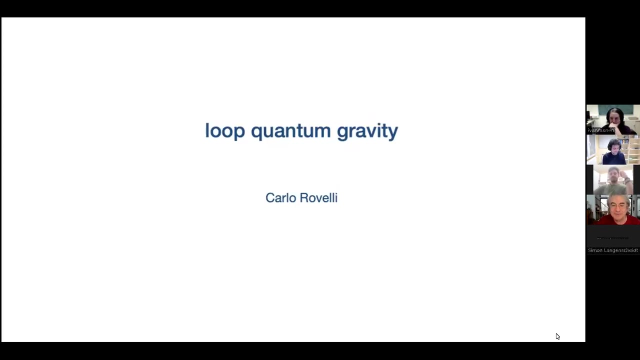 Very kind. I'm a horrible musician and I was involved in the in the in in the music, because they are the real musicians, are good musicians. So, yes, I'm going to talk about loop quantum gravity And let me uh, And so let me start by thanking all of you for this invitation. 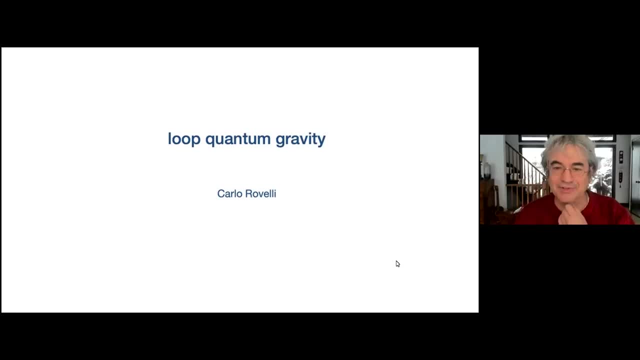 I know that mostly you talk about yourself, young people, and I'm the old guy, So I'll do my job as an old guy, giving you the way I think about loop quantum gravity. So this is not, of course, a class in loop quantum gravity. 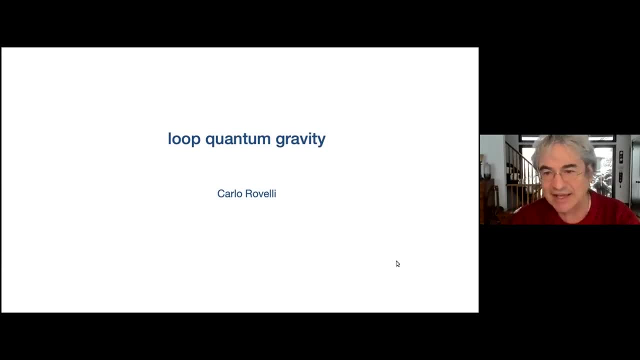 I'm not going to define thing and derive thing. I'm giving an overview Um the structure of the theory, why I think it's interesting, And then also at the end a little bit of sort of framing it in the context of other. 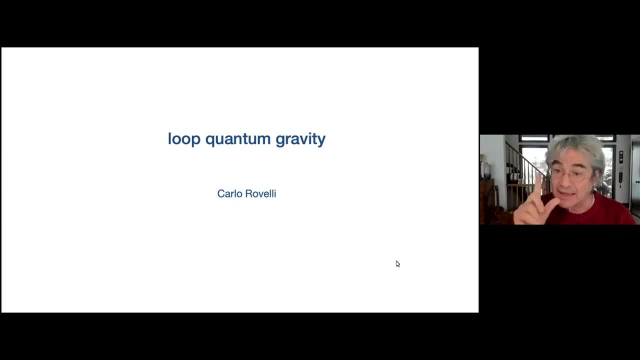 possible approaches to quantum gravity. Good, And if you have questions, do stop me, But at the end I will be. I have time. So if you want to ask questions, discuss also not just technical questions but also perspective things, general ideas, comparison. 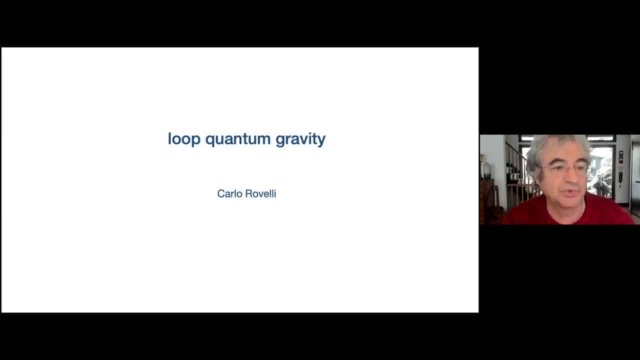 I'm happy to Uh, uh, so to to, to spend some time with you guys and uh, um and uh tell you what I think. Let me start by saying what is loop quantum gravity? because, uh, um, not all things that. 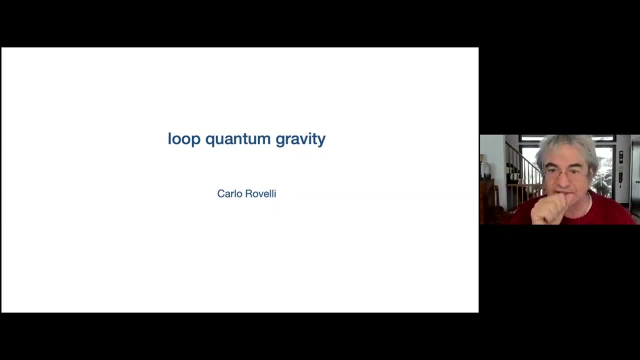 go under the name of quantum gravity, the literature, are actually the same research program with the same research aim. So, um, this is um what I think. uh, loop, quantum gravity is what it is in, in, in, in. 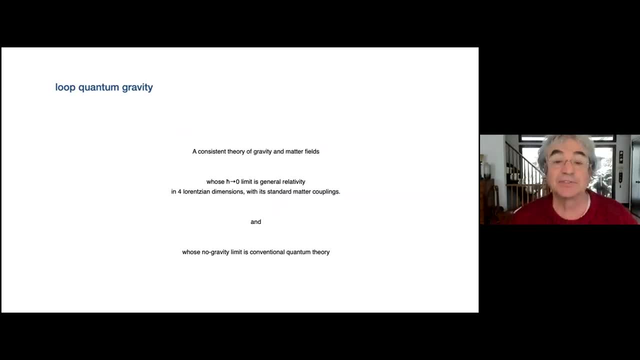 my mind. Uh, let me just read it. It is a consistent theory of gravity and uh uh, matter fields, quantum theory of gravity and matter fields. Um, who's uh uh H bar going to zero? The classical limit is, uh uh, general relativity. 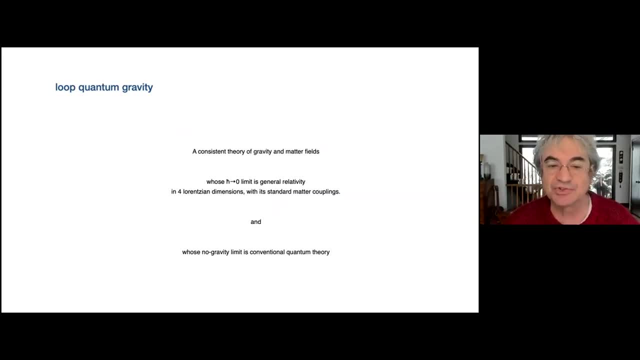 And by general relativity I mean the real physical one in four dimensions, Lorentzian uh, with its standard matter coupling Um, and whose uh non-gravitational uh limit is conventional quantum mechanics. Now this seems uh sort of neutral as a characterization, but I wanna uh, uh it's. 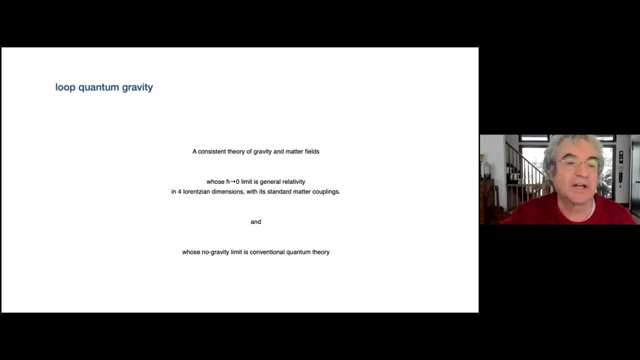 not at all. There's a number of points are important here, Um, the first is that this is a consistent theory, meaning that the claim of uh uh loop quantum gravity to be interesting is not that, um, there's a unique fixed procedure. 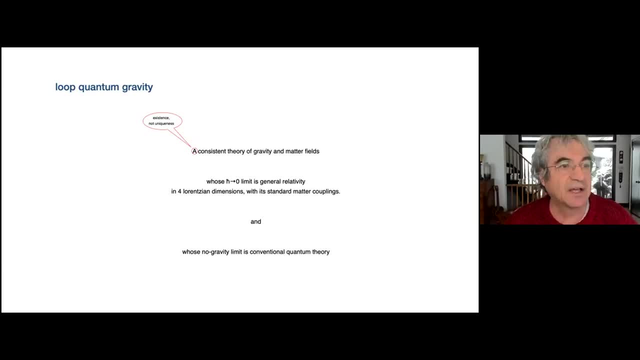 given a classical theory to construct a quantum theory. Uh, and uh, uh, so, um, uh, that's for sure the only possible quantum theory of gravity. Um, but it's the other way around. I mean, it's, uh, it's, uh, it's a century research for a half a century research for. 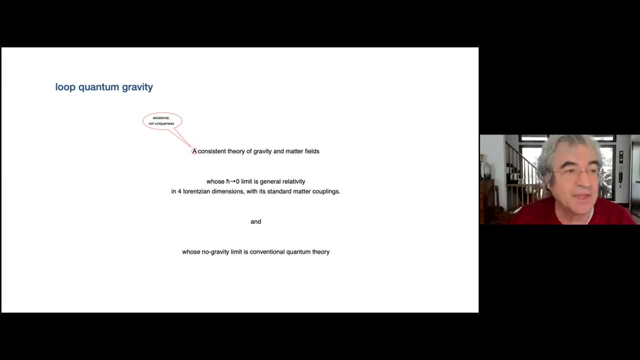 a theory of quantum gravity. It's very hard, Uh, it's not easy. Um, I think we don't have many, we have very little possible theory of quantum gravity. This is one possibility. Uh. so the question, uh, why is it defined this way? 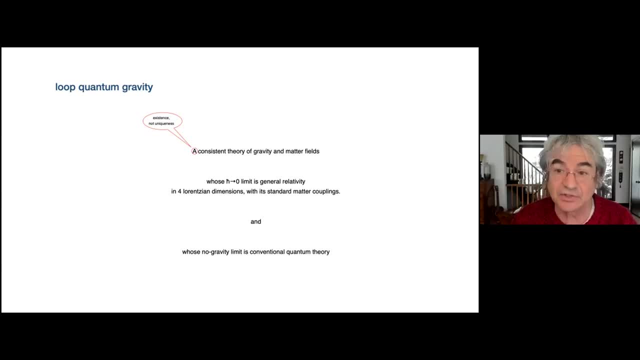 And not in another way. uh, it's not a good question, uh, with respect to the, to the aim of the theoretical research. It is a good question with respect to the empirical verification. I mean, if, if we happen to have more than one consistent theory, then we can ask. uh, 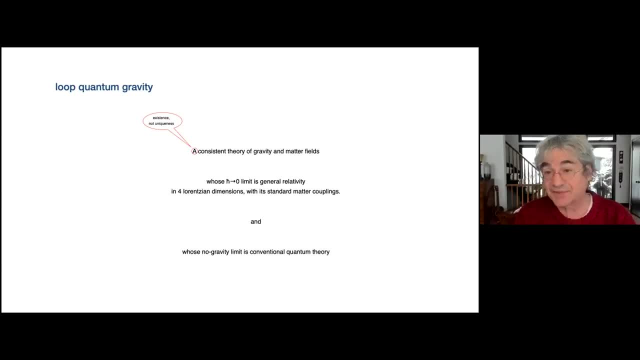 uh nature, with experiments, which one works the best? I mean we can find uh uh, uh, try to distinguish them empirically, and this it's going on. It's going on. So I will say at the end of the talk: uh. second point: uh, consistent means uh, both. 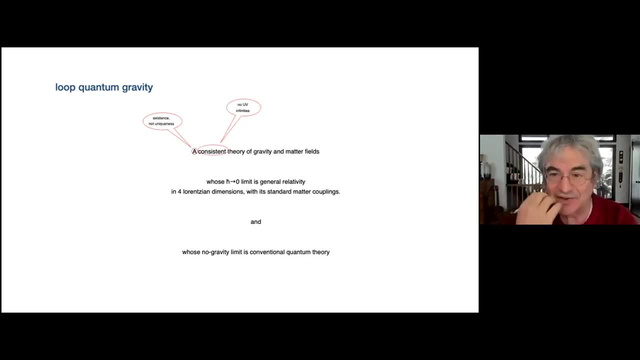 uh, coherent within. this is a well-defined mathematical formalism, Um, but also uh, that there is a conceptual way of thinking about that. What? how do we think about the quantum theory of gravity, What it is to measure space time? 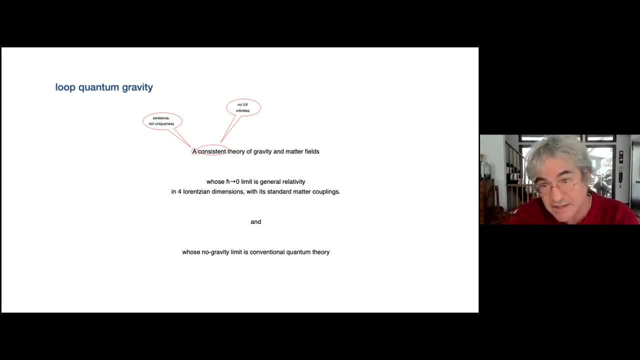 And, of course, consistent in the very simple sense that um perturbative quantum general relativity, done Uh usually by perturbing around the cosmic space, is inconsistent because, uh, the ultraviolet divergences, as you all know. 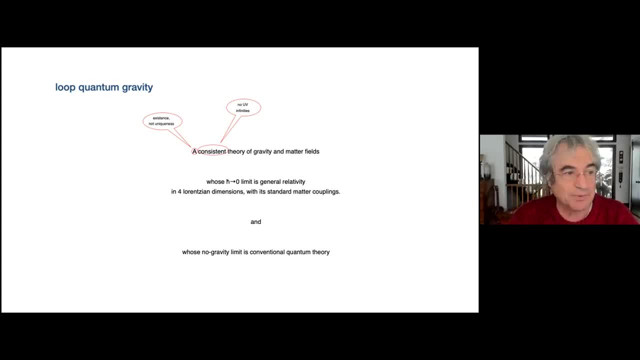 So the main point, the zero point, the essential point about consistency is that there should be no ultraviolet divergences. and look onto gravity. There are no into value divergences. Um, and he's also consistent in in the other sense. but the key, uh, key is what um next? 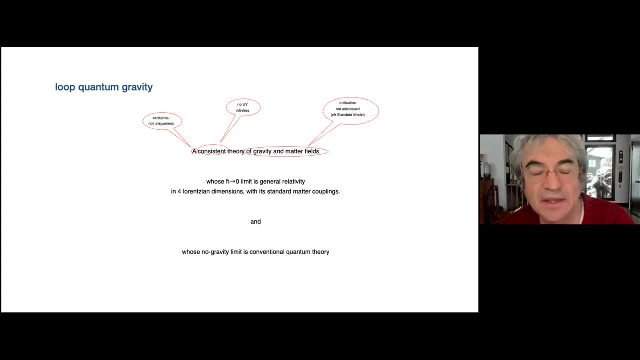 point. uh, it's, uh uh, a theory of gravity and macro fields. but careful, this does not mean that is a unified Theory. Um, the standard model is a theory of the weak and strong interaction. It does not unify the weak and strong interaction either. two different things, two different. 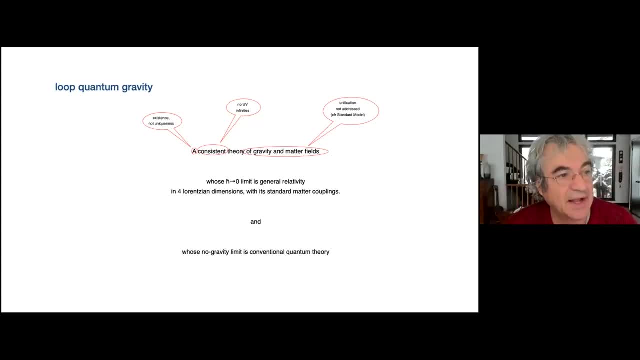 fields is a divine. the salon field and the glue on fields- Um, here's the same. It's not a unification. Unification is something else. Unification is the idea that there is a simple structure from which all the things we know in. 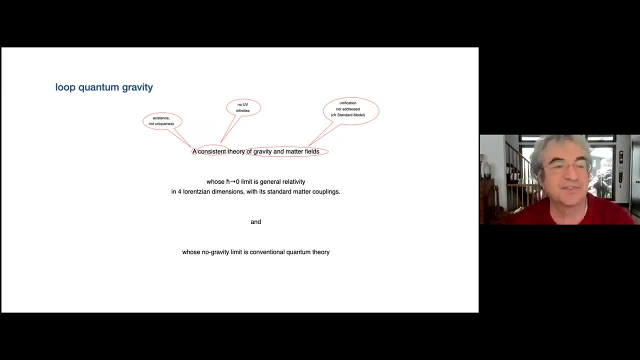 nature derive. I don't know string and everything is made by strings. This is not at all the aim of loop quantum gravity. My own opinion is that we are very far away from Having a unified theory of the world. Nothing has worked so far in terms of unification. 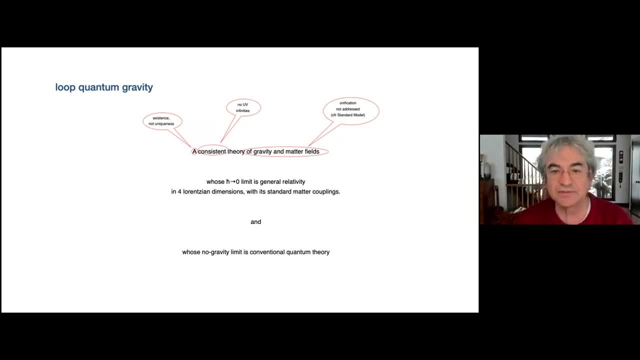 So maybe there is, but this is something for next generations, not not for us. It's a very specific problem which has nothing to do with unification, which is what happens when the gravitational field um has behavior that we cannot- uh uh, disregard its quantum. 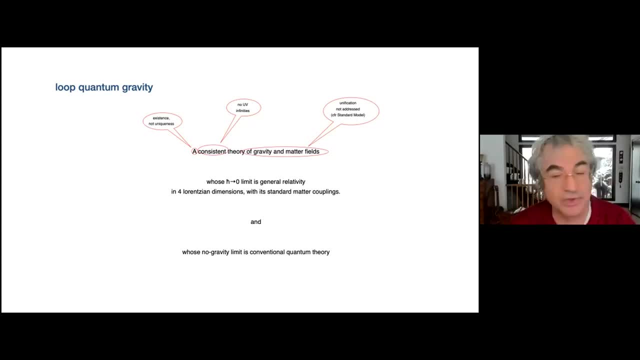 behavior, What happens saying to black hole? What happened at the end of the okay Evaporation? what happened at the big bank? the physical questions that um Involve quantum property of gravity, and that's what quantum gravity it's meant to um describe. 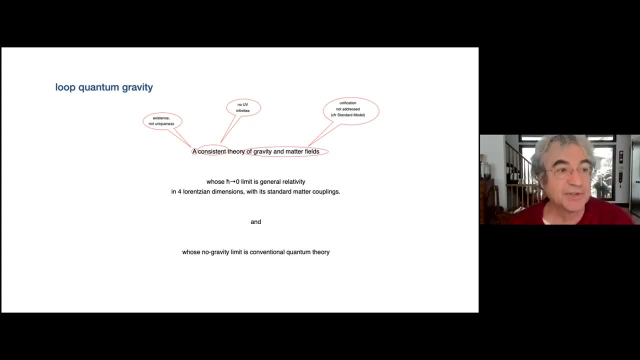 like uh. QCD is meant to define the quantum properties of the uh, the glue on fields and the strong interactions not to unify with uh, electro electromagnetism. Um, next uh is uh. I just want to stress that uh cinematic happening's only because uh uh you. 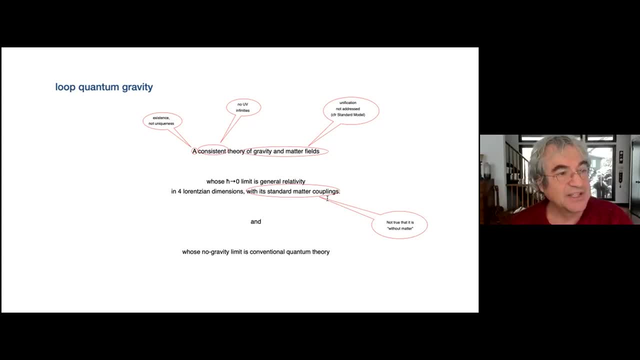 know there are play mix around and uh and uh. you often read that. So, Oh look, quantum gravity is only about gravity, pure gravity. Uh, the loop, people don't know how to do um, Matthew field. 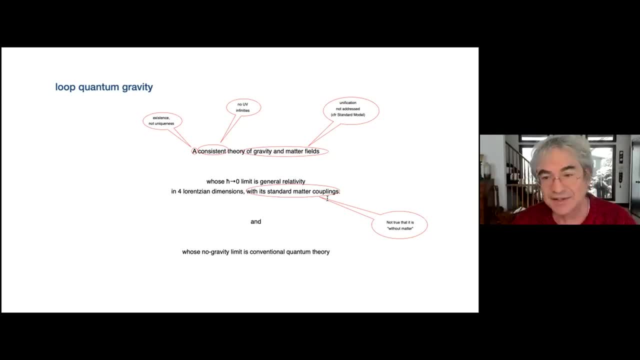 That's completely false. I mean, the people who see say that is people who started looked at loop quantum gravity 30 years ago and have never looked, uh, since. so it is, uh, the theory can be formulated with Matthew fields. 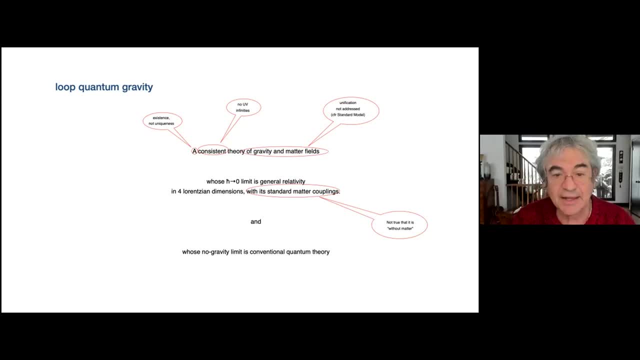 I will not go into the company with Matthew fields much unless you ask Um, but it is in the books. and then there's a subtle point which I want to um stress upfront, Because there's a source of confusion: Um is loop, quantum gravity, a quantum theory, a conventional quantum theory. 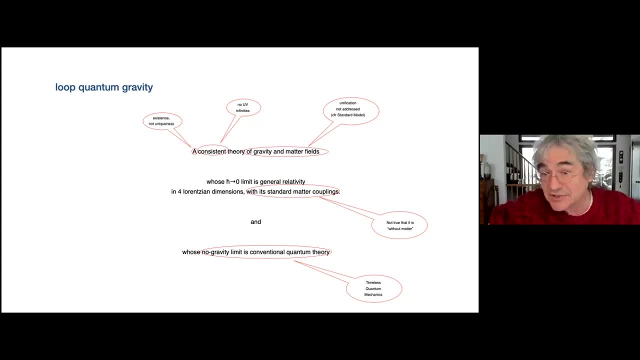 Well, depend what you mean by conventional quantum theory. certainly a quantum theory, but it's not conventional. If by conventional quantum theory theory you think, um, a theory defined with a shredding of the equation, with external time, that um, that, uh, that evolves, and there's a lot of people who, especially in the philosophy, 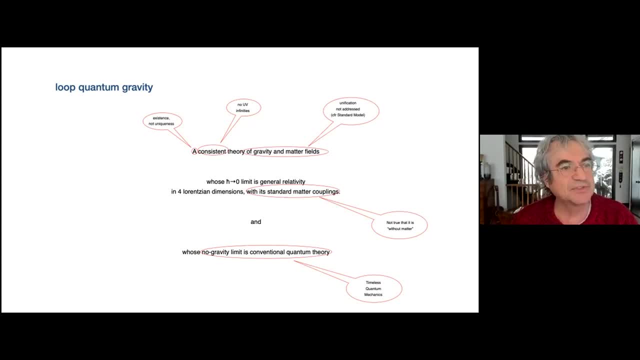 um world, but also, uh, a little, Some, some corners of a physical world. who says, oh uh, you cannot do quantum gravity because what we do is not the standard quantum mechanic, with evolution in an external time. Of course it's not, because general activity is not that way. 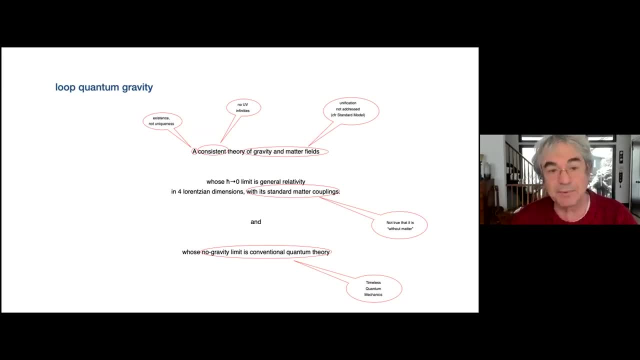 So, if you want, it's uh. strictly speaking, it's a generalization of quantum mechanics, um, which allows us to define, to describe temporality in the way generativity is, um, uh described temporality And which, in the, in the appropriate limit, is the standard quantum, uh, quantum mechanics. 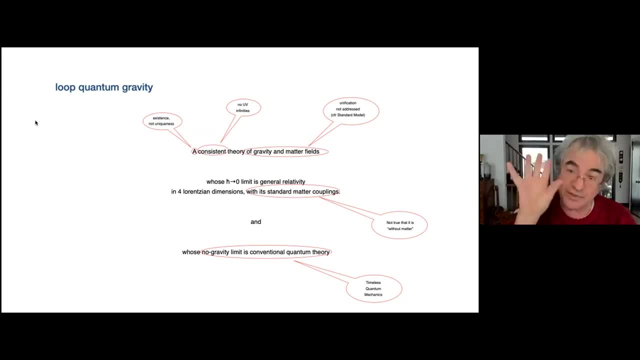 So this is, uh, what loop quantum gravity is. It's a consistent theory which has the two um, the two limits, as as we want. Now, how is the theory? What is the theory? The theory is, uh, the way you view it. 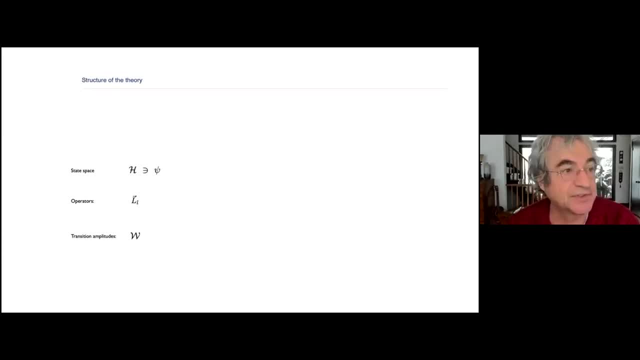 I mostly work in what is called the covariant version of the theory, not the canonical version of the theory, So it comes in two flavors. Uh, now is more than a decade that they work in the covariant version, So I'm going to talk about that. 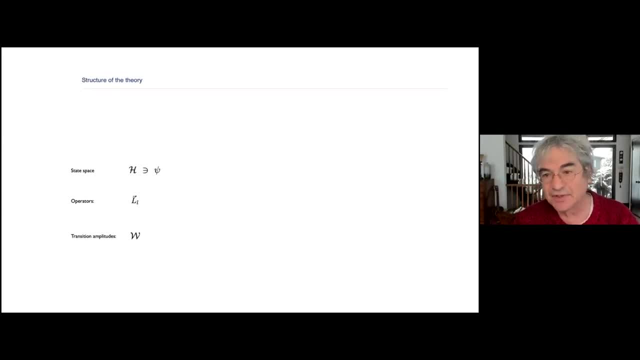 Um and uh. the structural theory is, uh, is is pretty much the structure of a standard quantum mechanical structure. Think at your preferred quantum mechanical model. where is uh QED, or the harmonic oscillator, or, or, or or the hydrogen atom? 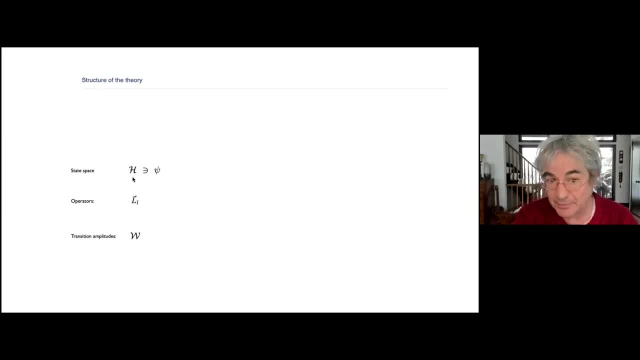 There's a state space, um, which is a Hilbert space, in which there are vectors which you write psi or uh uh represent state. in some sense It's a bunch of operators that represent um, describe the kind of thing we can measure. 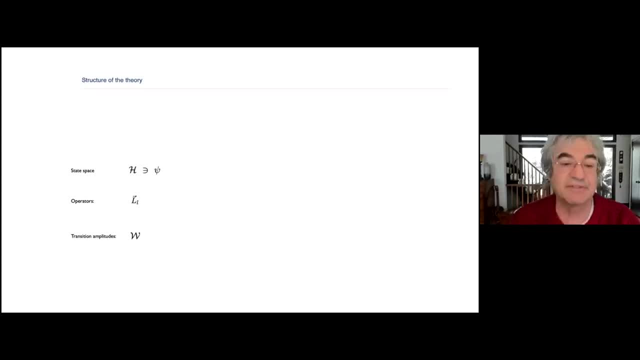 So when we interpret Track with the system here we interact with space time, with gravity. Uh, we can measure things. We can measure the gravitational field- Uh, we do it every time, LIGO- measure the gravitational field. but also when you measure distance, you measure the gravitational field because it's the integral of the square root of Jim, you knew. 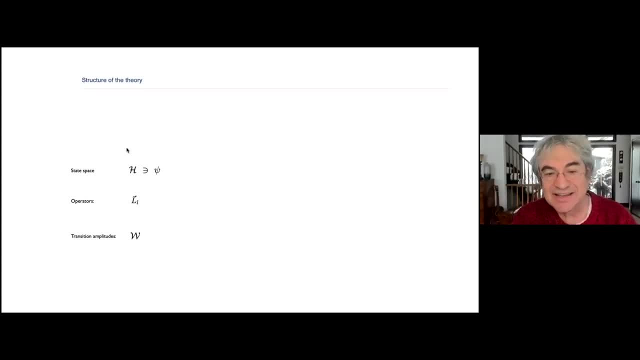 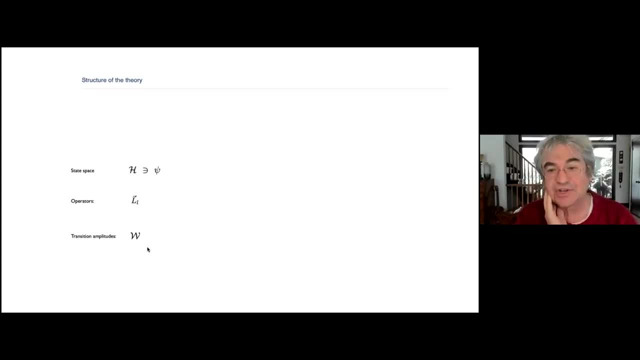 And the dynamics is given by giving transition amplitudes, So it's not given with a um. Hamiltonian in the covariate formulation, is given by giving transition amplitude, not a Feynman, If you want. You have a uh, the, the, the, the, the amplitude going from one point to, from one value to another value. 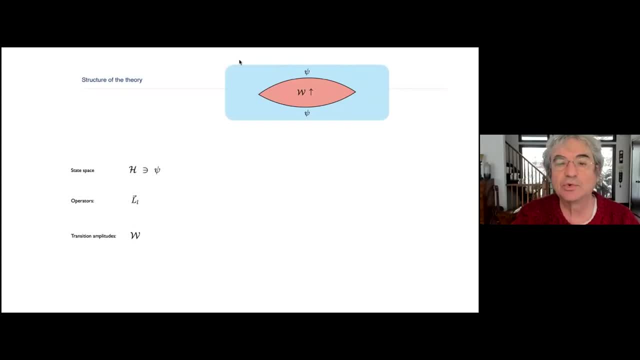 But cancel. These are not strictly Speaking. quantum gravity is to this blue is a space time region, so let's say that this is space, in this, in the horizontal direction, in time, in the temporal direction, and what we want to describe with loop. quantum gravity is a process, this red area, a process which is limited in time and 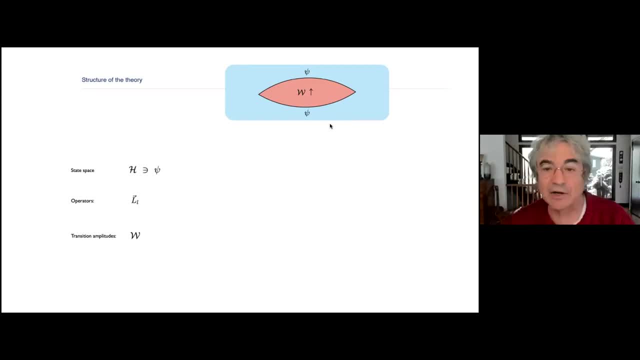 limited in space. so think, for instance, a black hole that forms, goes through some quantum stuff and whatever happened next? okay, so the amplitude to describe this process and the states are the boundary of this process. so at the beginning and the end and in general activity, this boundary, 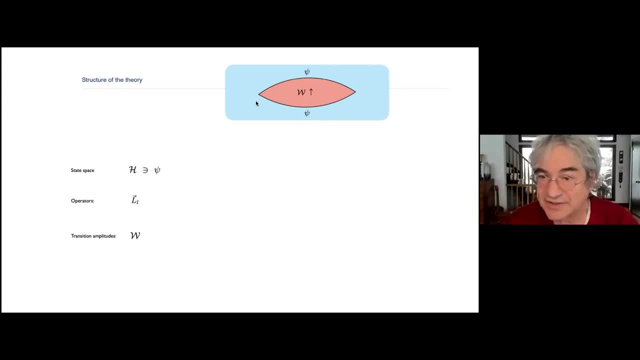 don't need to be a constant time surfaces. in fact there's no meaning, no, no, no, no sort of objective meaning in constant time surfaces in general activity. so the clean way to think about that is to take surfaces uh, which close, is a finite space-time region and it's convenient to take this uh surface space-like and the quantum. 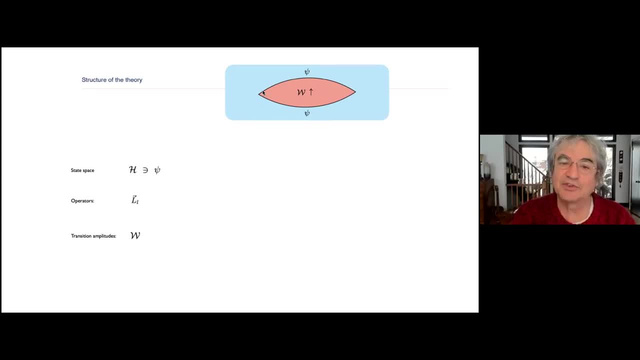 state is just whatever is at the beginning of the end of the process, which means if you think you are so, think quantum mechanical. this is the quantum system. and outside the quantum system you make measurement before and after and you compute the probabilities associated to possible set of outcomes. the relative probability and the state can be either thought as initial. 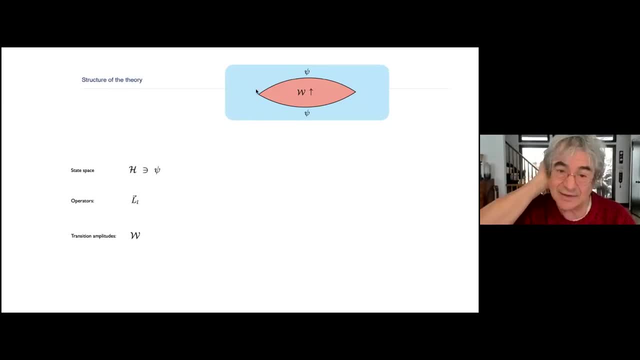 state on a final state or, as it is convenient, um, just mix the two, sort of take the tensor product of the initial and final hilbert spaces and view the state as the state all around it. now the key point is that in gravity time it's one of the variables, uh, that to measure at the 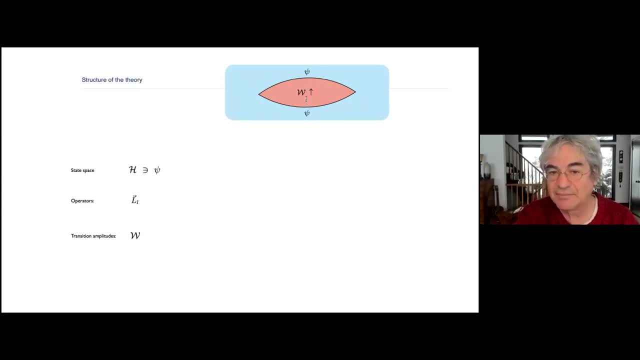 beginning of the end. so if you one clock, it will have some value at the beginning, one value of the end. if you have three clocks, uh, they will have have their histories and they will not give the same value, because in generativity, clocks uh do different things depending on what. 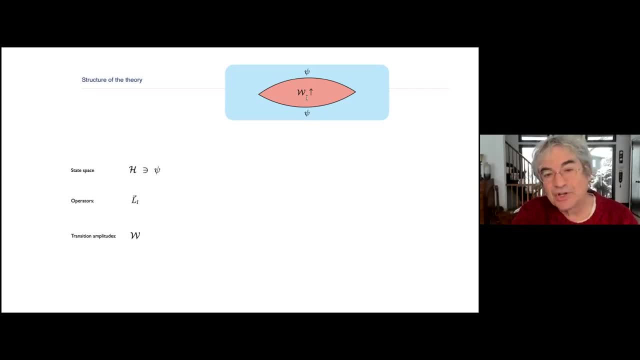 what happened to them. so this process is not uh labeled by an external time variable. the time variable is one, is, is is one of the um, uh, it. the time variables plural are uh. among the observables that you can measure on the status among these operators here. good, so the next thing to have. 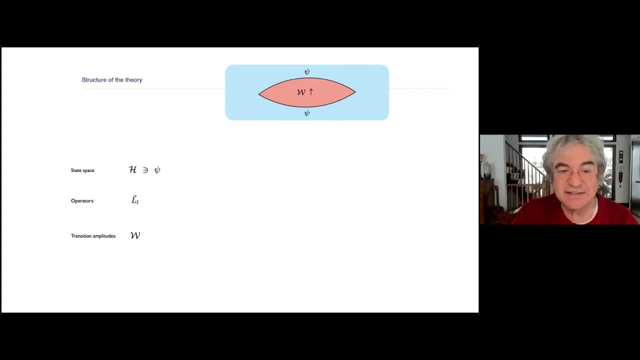 clear to understand loop quantum gravity is that the theory is defined um via a sequence of truncations, plural um. why? well, this is uh very much like in uh quantum field theory. in fact, in quantum field theory we always do that. if you think a lattice gauge theory, that 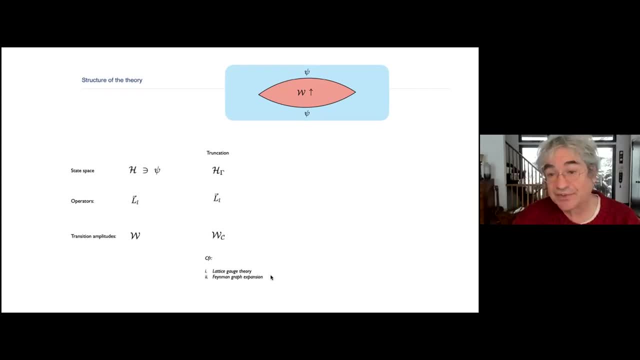 we have two good ways of defining quantum theory. one is on the lattice and one is a thymian um expansion with the final grass, and in both cases, what we describe it, what we have, is a, a sequence of truncations. uh, with a lattice, we define the theory on the lattice and then we 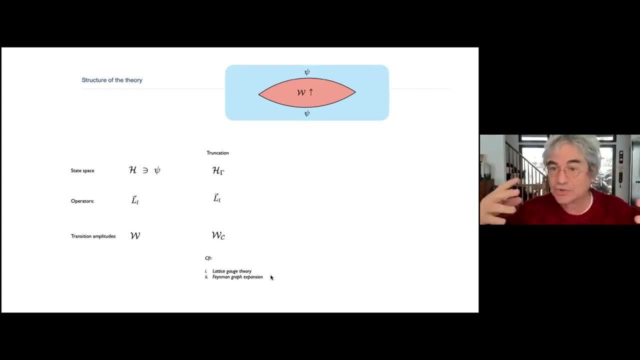 in some sense we say that the more the lattice is the reach, the more you capture nature, and the final graph is the same. you have, uh, you compute the transition amplitudes, uh summing five and graphs, and the more you sum uh, the more you have uh well-defined transition amplitudes. but 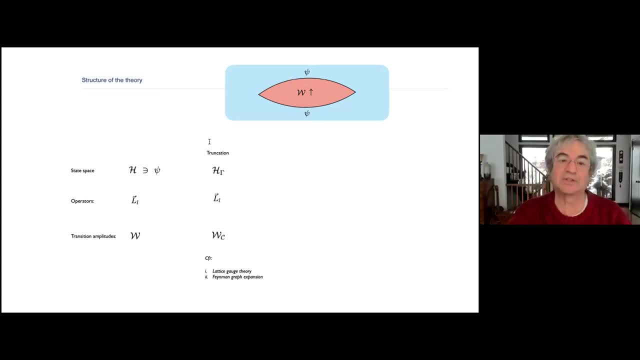 we always work with truncations and so we do in, in, in quantum gravity. so we have a family of Hilbert spaces that increase the truncations labeled by some gamma, and one can do some fancy math, but in some sense the full Hilbert space is the limit of that which. 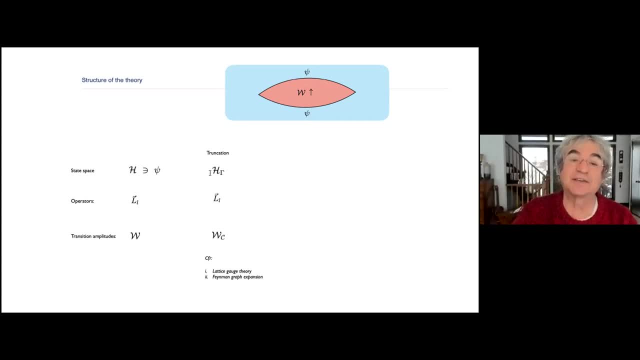 can be done with some fancy math. the observables are defined on this truncated Hilbert space. i'll tell you in a moment what is gamma and the transition amplitudes are defined also with truncations on the same boundary of the space. you can have more refined. 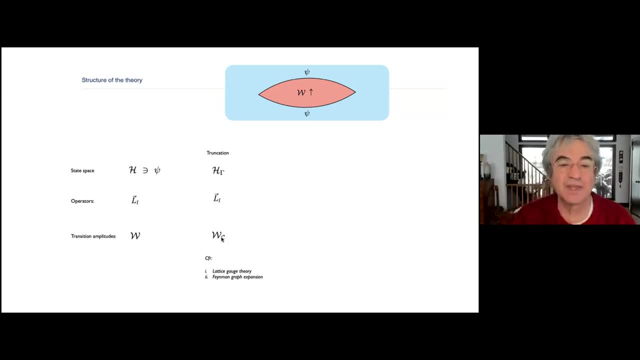 uh, more and more, uh, better approximations, um, with refining the truncation. now, what are these truncations? well, the beauty- and i let me just say i want to emphasize the point, like the beauty- is that, uh, you can think either that what is going on here is like lattice gauge theory, or that is. 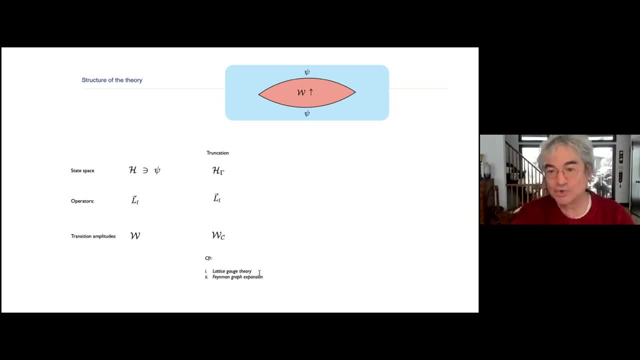 like Feynman graphs, and because we are doing the quantum gravity, the quantity of space-time itself, the two things match, the two become the same. let me show you the truncation of the uh of the states. um is labeled by this gamma, where this gamma is a graph, a set of the combinatorial structure given. 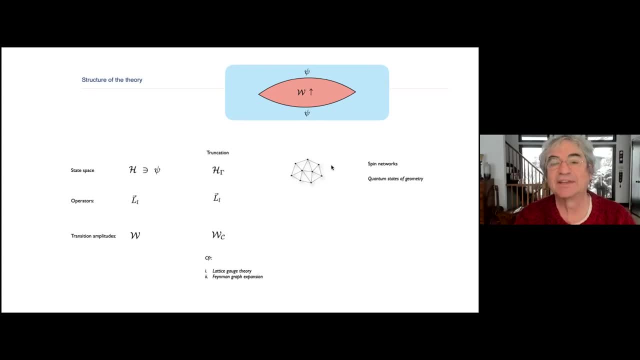 by a set of nodes, of points and and links, nodes and links. okay, and one way of thinking about that is that each point is a, is a point in space, and the links say who is next to one another. so this is really a truncational space, like in lattice gauge theory. 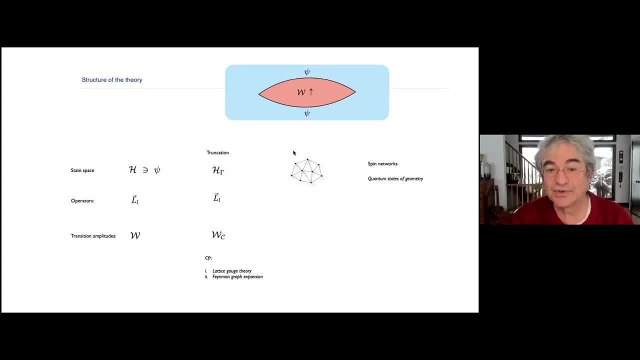 is exactly what we do in when we discretize the quantum theory on. on lattice causes a discretization because instead of any number of degrees of freedom, you have a finite number of degrees of freedom there. okay, i will come later to a point in which there is a key difference in in between. 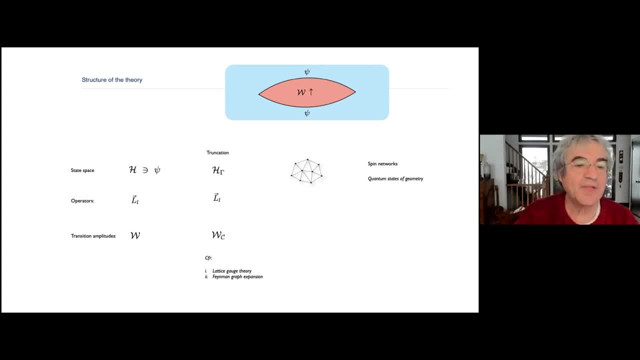 lattice gauge theory, but so far it's exactly the same thing. and then the uh, um transition amplitudes are also described with a discretization. it's called c. now where c is um, you can think as a four-dimensional distribution, and then you can think of it as a four-dimensional distribution. 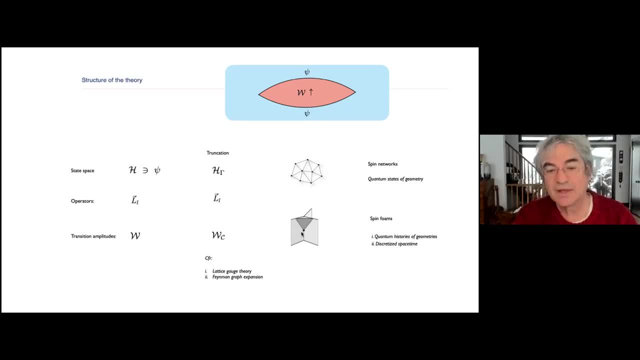 and then you can think of it as a four-dimensional distribution: uh, the points and um, uh links, which are called edges in this car in this time, and then there are also surfaces. and one way of thinking about that is that this point here is a vertex. it represents a bunch of a piece of space time. 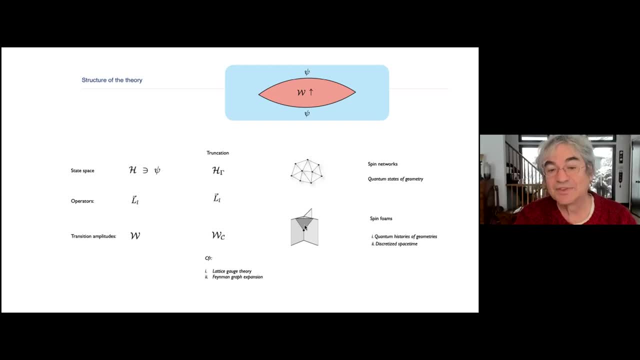 and two space times are connected next to one another. when there's an edge between between the two, and a set of- uh uh- space times can, can enclose a two-dimensional region which is dual to the surface. here, um, what i'm saying is that this can be viewed as a discretization space. 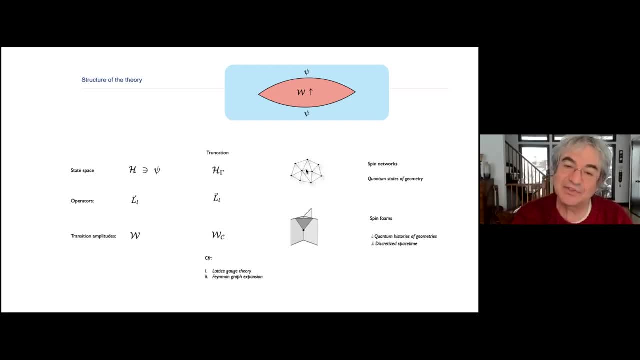 time, but can also be viewed as a history of the states defined on a um, on a spin network. so if you on on this graph here, so um, this line in time is the history of a node, the, the, the surfacer are the history in time of a link and then the this uh. 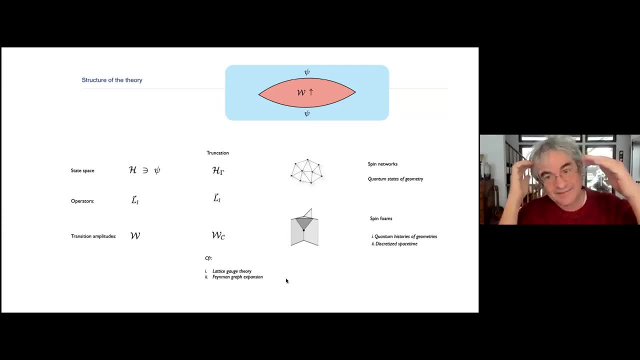 discretization is really like a Feynman graph. so a since we're doing quantum mechanical space time, the discretization space time is a history of the discretization of the bound. now the actual series is given by defining mathematically the silver space, this operator, 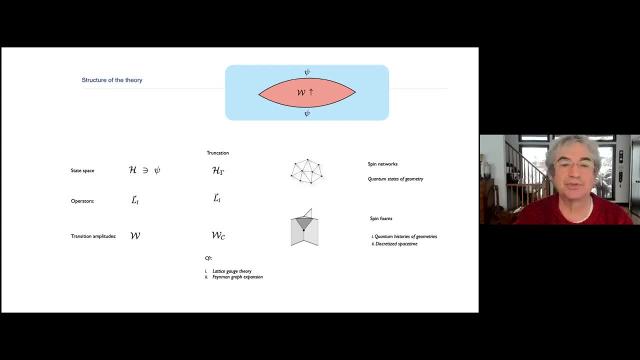 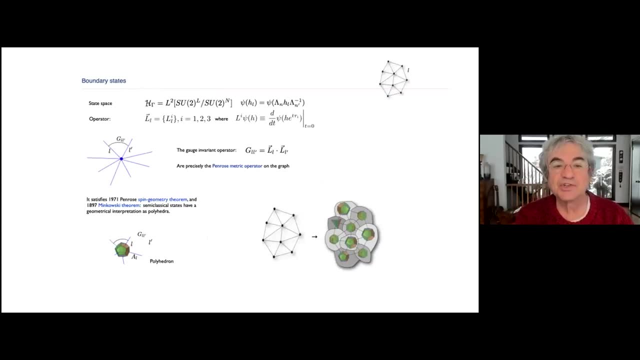 and giving expression for this uh uh transition amplitude here. so let me give you a little bit of details of all that: the uh Hilbert space associated to a uh. one of these um uh graphs here is uh, something that, if some of you are familiar with, Latte gauge theory- is exactly uh, like the Hilbert space of a Latte gauge theory, of an SU Latte gauge. 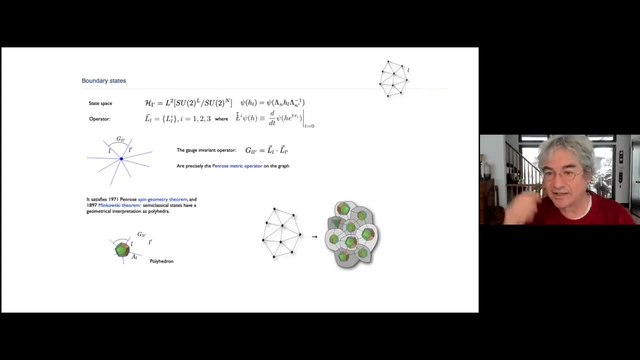 theory. uh done, uh, canonically Wilson-Cogut, if you have studied the uh Latte gauge theory. so this means that the states psi are wave functions of variables which are associated to the link. there is an SU group element for each link, uh SU group element called little h. so h sub l? um it's. 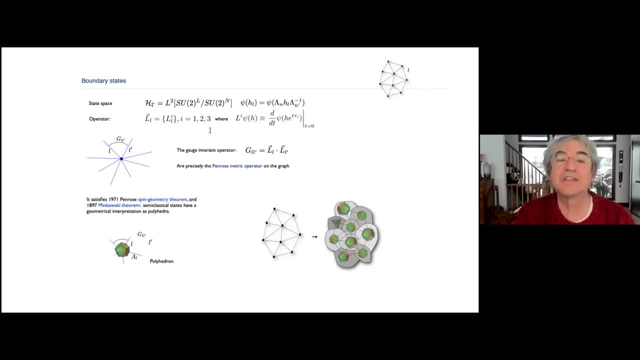 it's a. you have a SU group element of 3a to each link and the. the quantum state is just a complex functions of all that, um, with a symmetry which is related to the gauge, symmetry at the, at the nodes. I'm not going, I don't want to go into the detail. and then there are some operators which are the: 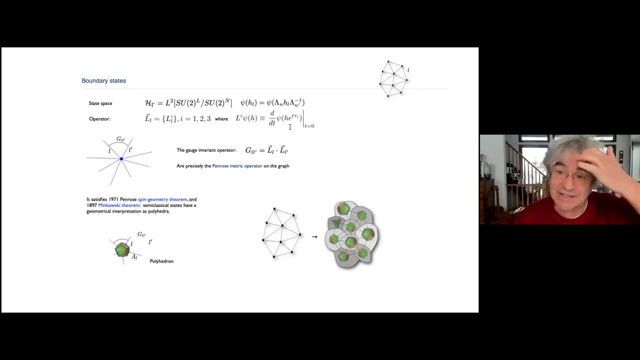 natural operator that you define on this kind of things, which are in Latte gauge theory, would be the metric field in the direction of the links in gravity, are just the geometry, because the, the, the operators have the thing that in the classical limit is the metric. so pieces of geometry and uh. 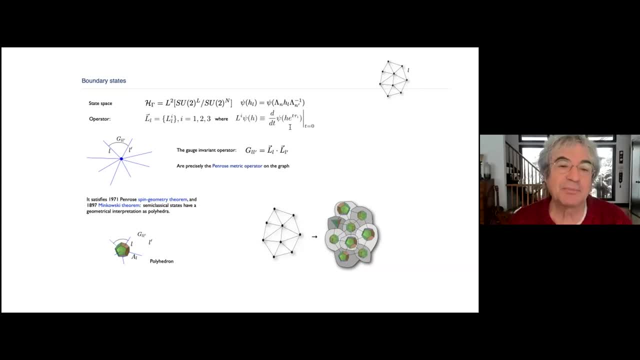 I'm not going to detail, but this is a beautiful piece of mathematics, because um these operators can be obtained as a quantization of the gravitational field: uh, g, mu, nu, or more precisely the tetrad. uh, the square root of g, mu, nu, or more precisely the triad, which is the gauge fixed at. 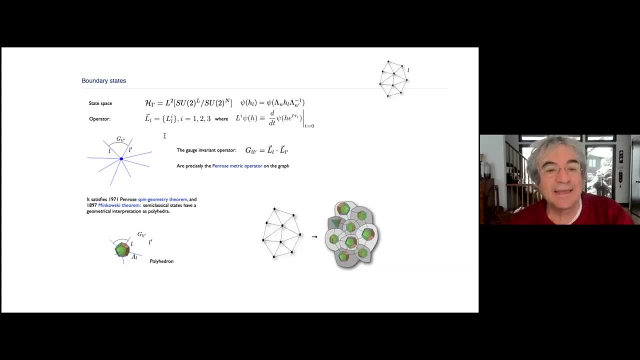 the position of, of the, of the metric, and this operator here satisfies property um. that make them exactly uh Penrose metric operators, which are the. the way Penrose um, back 30 years ago, constructed a quantum theory of geometry on graphs, in terms of operator of this uh sort here: 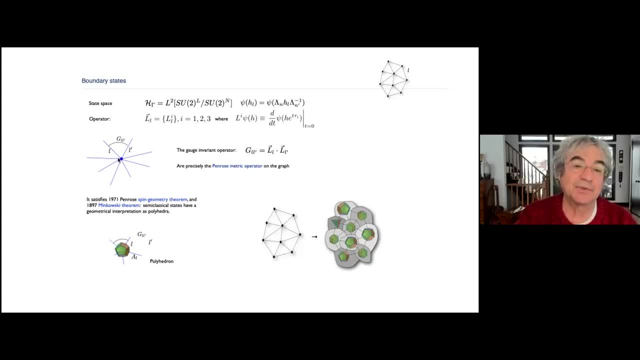 and the set of operators is written a little by links, by by link. so on a note, on a link, there's one per per each link- and a set of operator around the node um have a property, uh, but from their definition that characterize them as a quantity, that define the geometry of a polyhedron, so what? 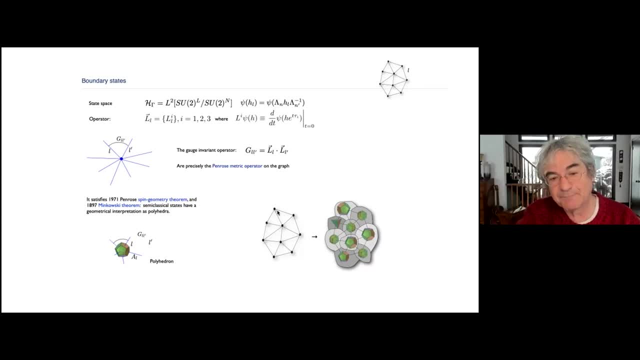 you can think about this uh uh uh graph here is that these operators here give it a geometry and the geometry is like giving a lot of polyhedra, say a tetrahedron or a more complicated uh uh geometry outside. so you this, this riddle, give, give a geometrical um. of course each one is flat, but the way you put, 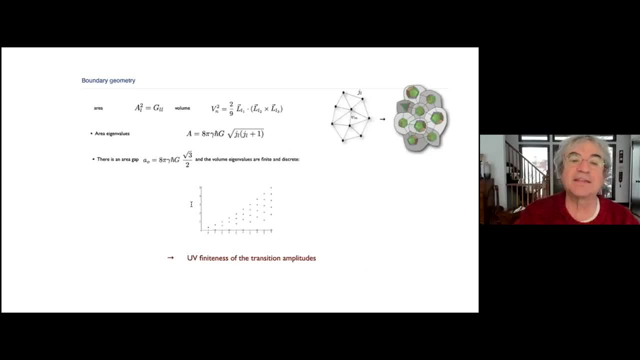 together you can get curvature, um and uh, the from those basic operators you can construct the geometrical quantities, the volume of the things here and the areas of the surfaces, defining this now. so far, all i've said about discretization, about polyhedra, is just a. 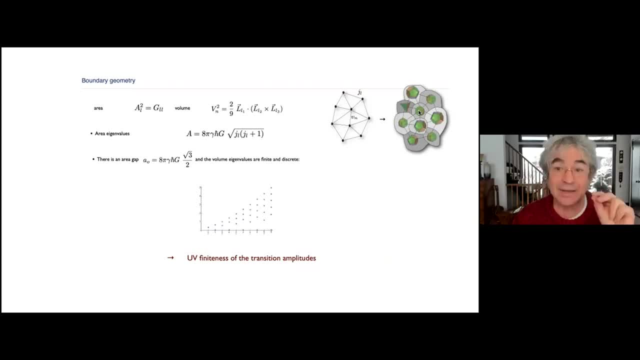 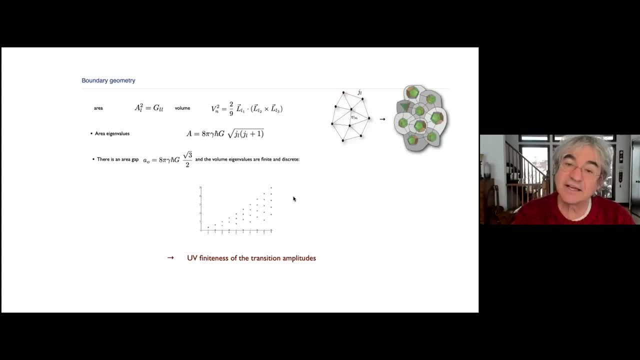 mathematics, which means that in each discretization, whatever you discretize, you always have a minimal length, a minimal area, a minimal volume, which means that this, as a quantum description of geometry, predicts a minimum size of anything. okay, minimum area, minimum. 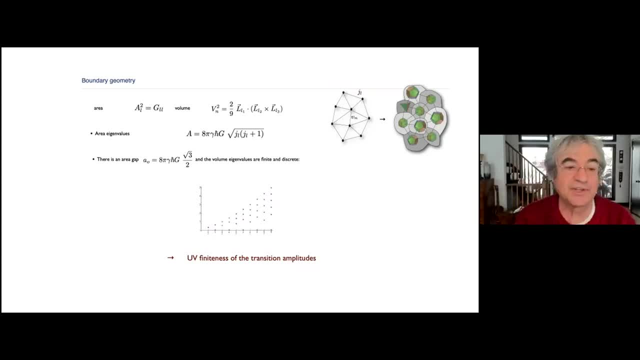 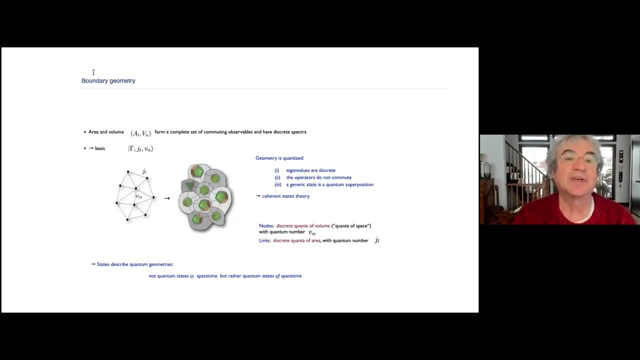 volume, And this is a root of the ultraviolet finance that we will see in the dynamical part. So let me just close this kinematical part. There is a set of states the Hilbert space admits, a basis which is obtained by diagonalizing area and volume. it's called a. 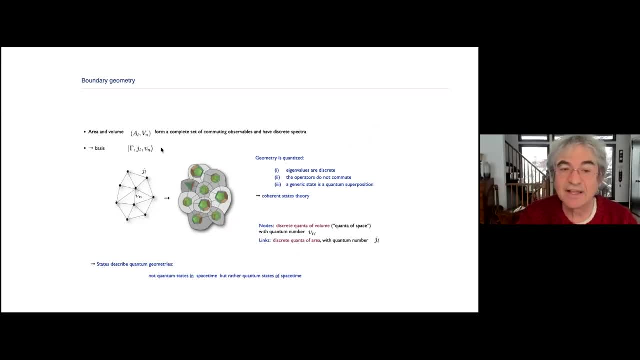 Spinnaker basis. it's written this way. here it doesn't matter where area and volume are discrete, but one key point is that take a tetrahedron. here the tetrahedron has one volume and four areas, and these are a complete set of operators- can be diagonalized. there are five numbers. 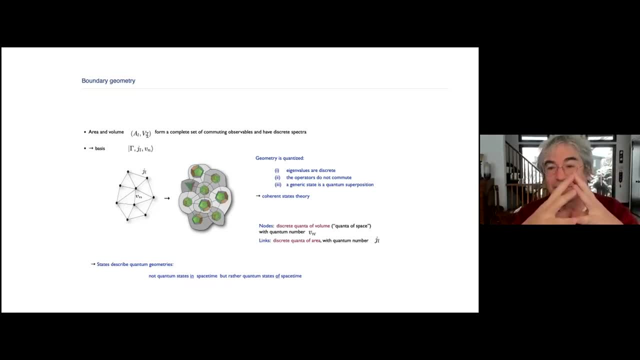 Tetrahedron classically has six variables that characterize its geometry, because each length you can make it longer or shorter. So what is missing? What does it mean? That you cannot sharply in the quantum theory have a value associated at all six levels. So you can't. 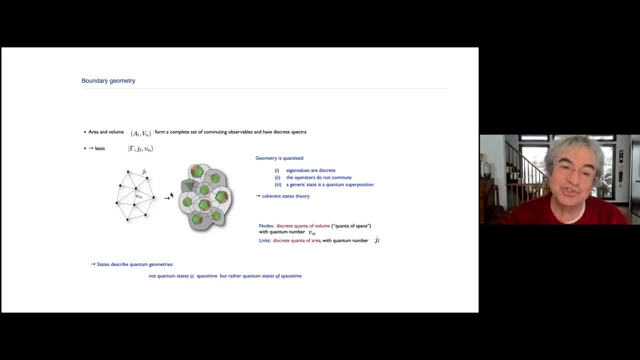 do this by disciplining this theory to estimate the number of Pediceless quantities. it's like angled momentum theory. So therefore the geometry is fuzzy in this mode. So you see, it's a standard quantum theory. Even values are discrete operators do not commute. geometry are fuzzy and the 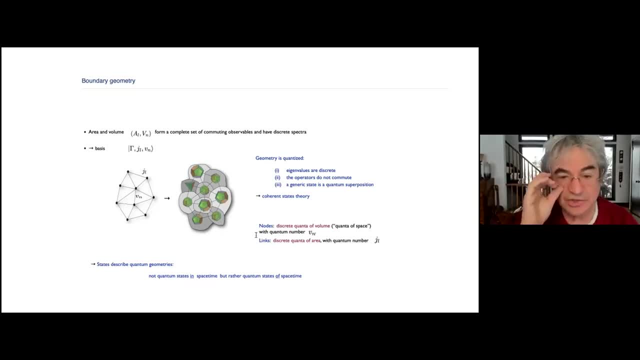 generic state is a quantum superposition of these things. This is the quantum theory of three- dimensional geometry. And last key point: these quantum states are not to be falanth to quantum states in space. they're at the quantum state of space itself, with, with a general 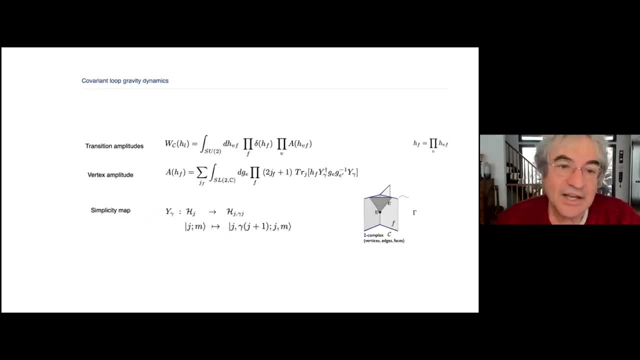 motion. So when we go to the quantum states are not to be вы😱😜d. ofaxial degrees, crabs s'sh it. Now let me go to the transition amplitudes. The transition amplitudes have a long story. 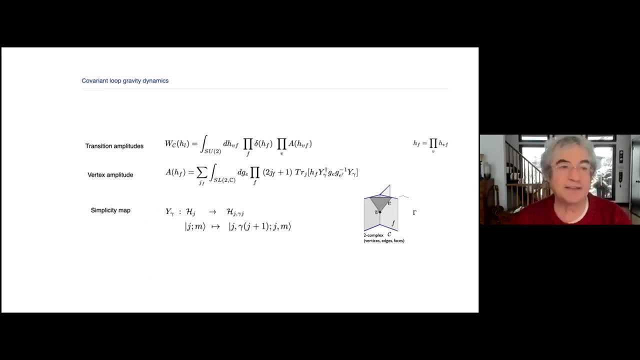 because there have been a number of attempts to define them through the years, with the sense that there was something wrong all through the years until this definition was found here of the transition amplitudes, which was obtained in different manners. One way of obtaining it is just through a discretization of a Hale-Einstein-Hilbert action. 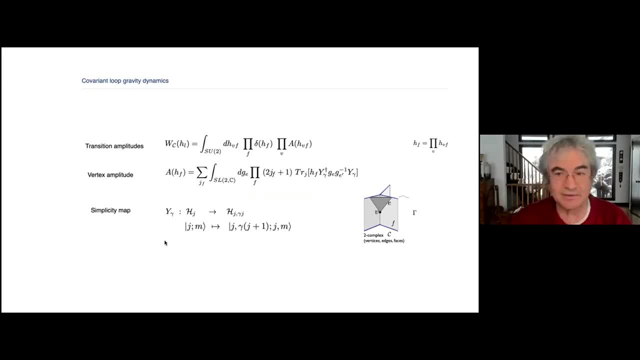 One way of obtaining it is through a canonical quantization and implementing the constraint in some way. It's a long story But finally given some states on a boundary. so on the initial say and final states, and remember the state of functions of SU variables. 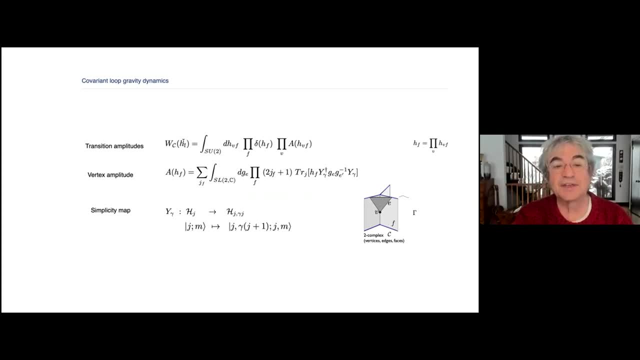 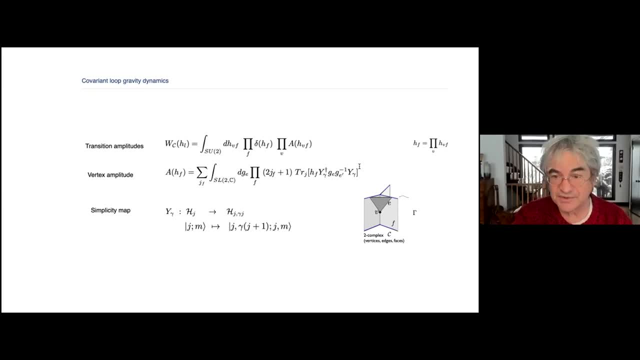 This is a definition of the transition amplitude which has all the properties that one want. It's very similar to gauge theory. You're integrating on internal variables which are both SU2 and SL2C variables. There's a vertex- amplitudes which 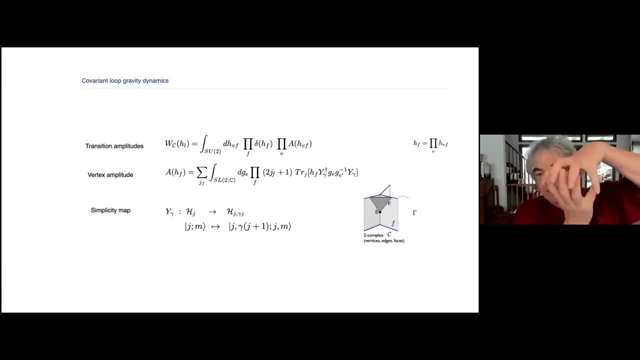 is the only non-trivial part of the story. So, to every vertex, every piece of four-dimensional spacetime, there is an amplitude which depends on the variables around it, which is a relatively simple expression which I'm not going to define explicitly because it's 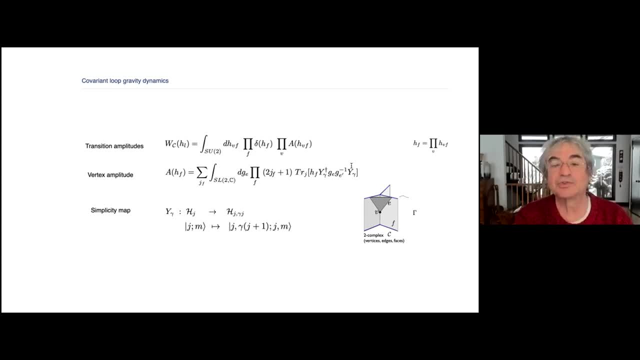 written in terms of representation: infinite-dimensional representation of SL2C. This is a trace in a certain representation of SL2C And the core of the mathematical theory is a map Between SL2C representation and SU2 representation. it's given in a canonical basis. 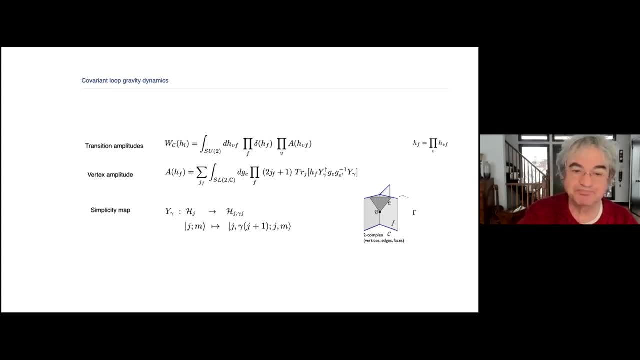 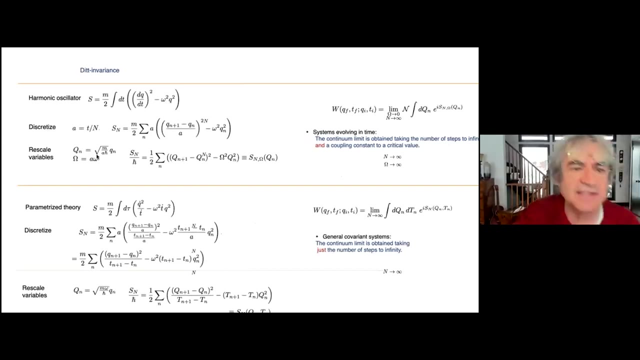 So there is some mathematics to learn to know how to use this thing here. But everything is well-defined And the key result of all that- oh sorry, that's not what I wanted- is that everything is finite. Now I just want to. I added this slide here. 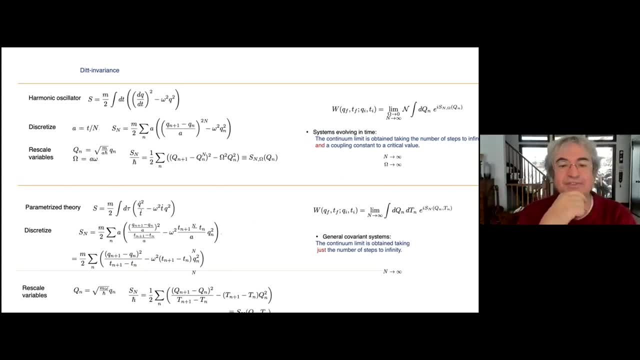 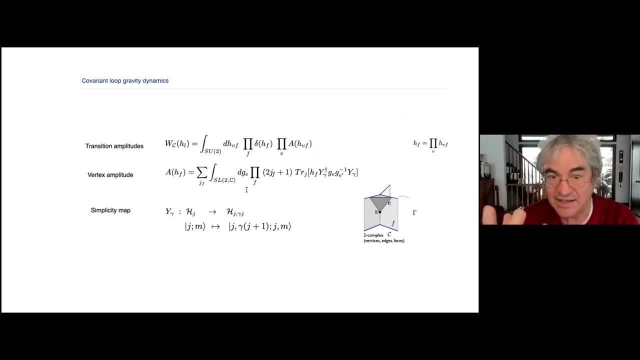 I don't want to go through. I want to bore you with math. This is actually very simple. but to tell you why this works And why this works, I mean why this definition here of the transition amplitudes actually gives something finite as it is, without any further limit. 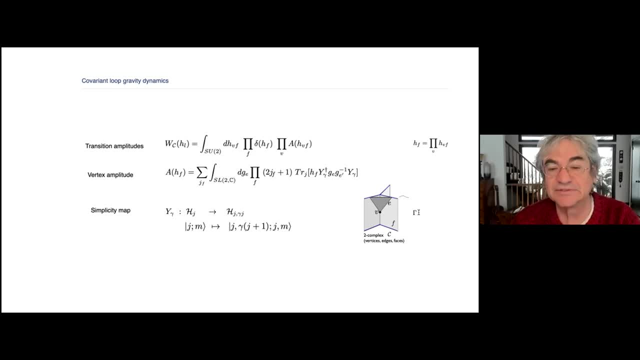 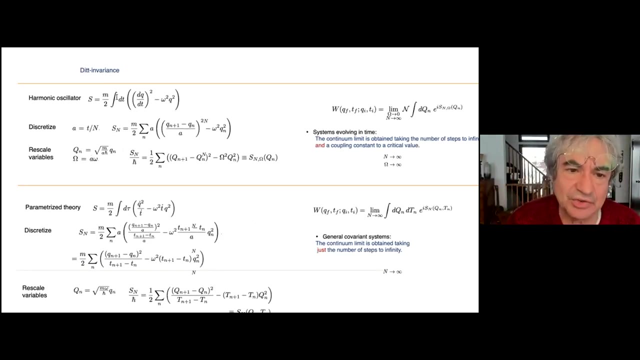 The only limit is that you can define the four-dimensional triangulation, You can change the C, And there is a reason in that, which is the following: Just one technicality, very simple, but in my opinion this is the core of the story. 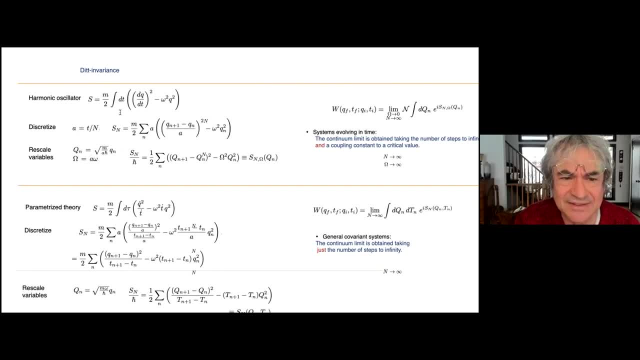 Take an harmonic oscillator. This is the action of an harmonic oscillator. Discretize it And you introduce a lattice spacing A And write the path integral. Now it's convenient to change variables from A to omega, which is just scaled. 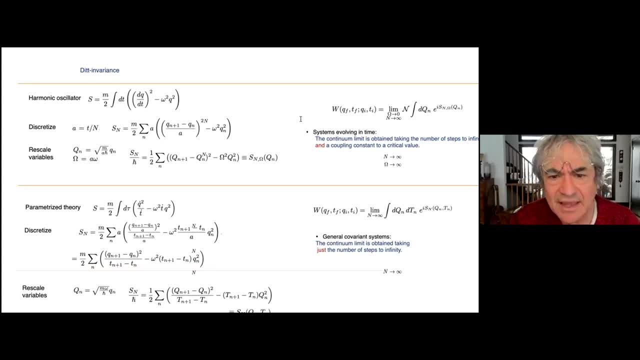 It's big omega, which is just the frequency scaled by A. And then you show that to get the actual transition amplitudes from the discretized parts integral, you have to take two limits: You have to increase the number of steps. 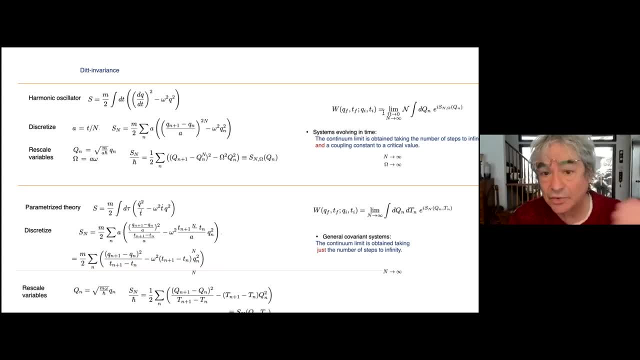 That's your discretization, this N, And go on a critical point. as everybody knows, OK, in quantum field theory you have to go on a critical point, You have to take a limit of something And when you do, discretization to recover. 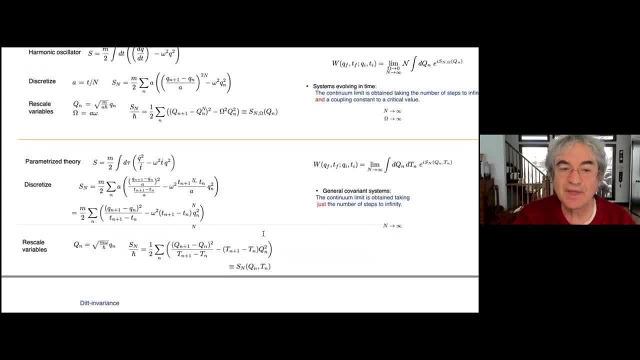 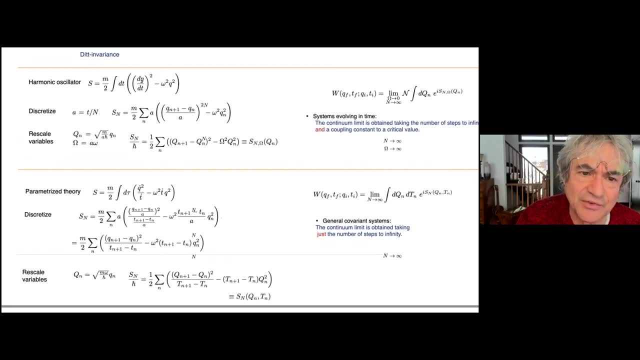 and the continuous theory. you have to go to critical point. But now take the same harmonic oscillator but write it in a discretized form. So instead of having a variable q, now you have two variables, q and t. You promote t to a independent variable. 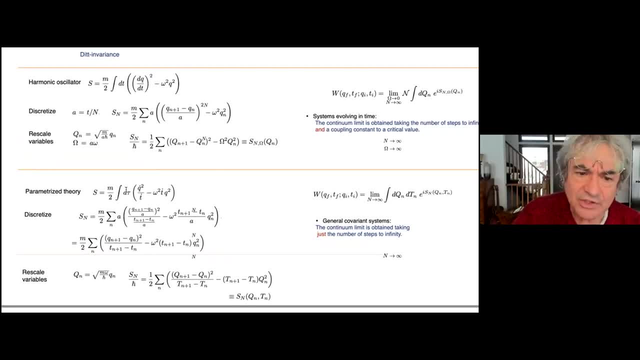 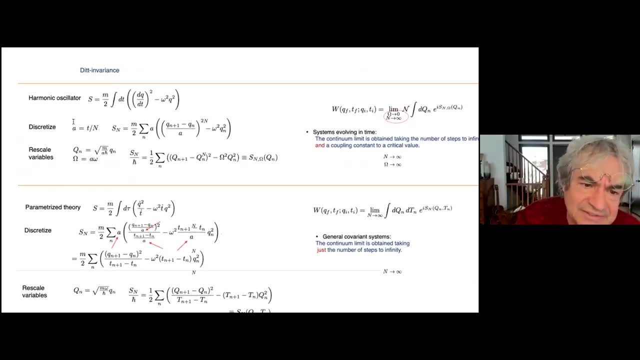 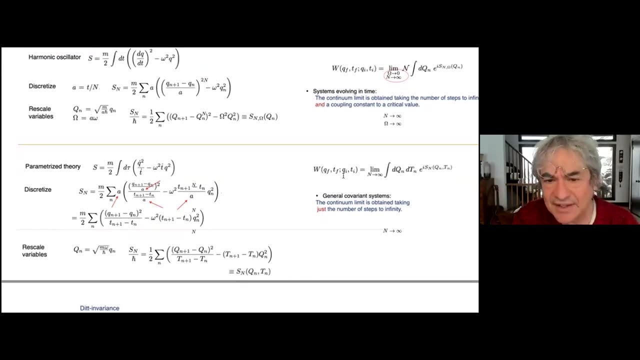 and you evolve in a tau which is unphysical. You do the same game and something absolutely magical happens, which is the discretization. the lattice spacing disappears from the action, So the same transition amplitudes can be computed without going on a critical point. 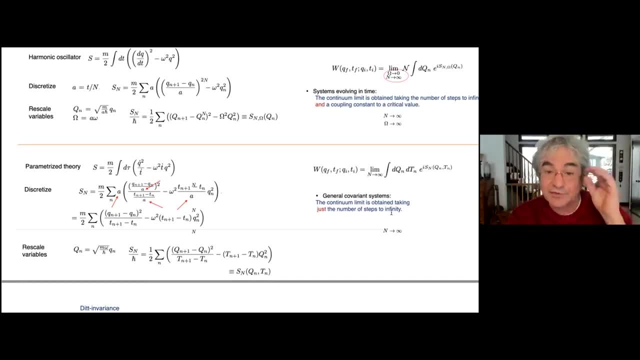 just by taking n to infinity, And this is general. If you do the discretization correctly, you can recover the physical transition amplitudes harmonic oscillator. we know what these things are without the need of going to Critical point, just by increasing the number of steps. 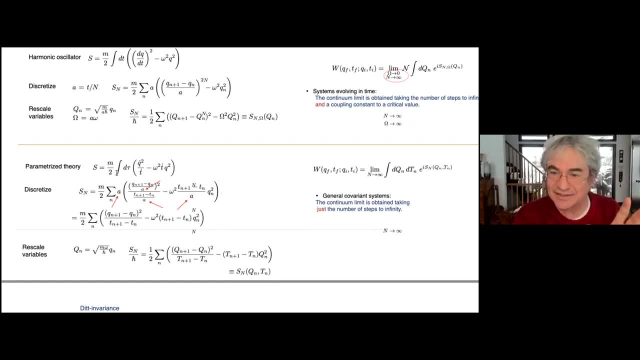 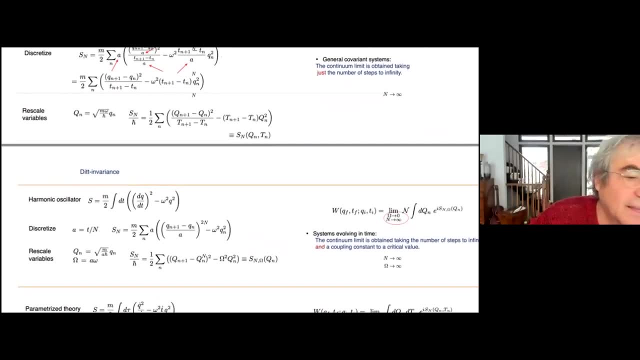 And that's why general relativity, which is a parameterized theory, doesn't need to be on a critical point, And that's why the transition amplitudes that I gave you before work and are defined as they are. So this was the definition of the theory. 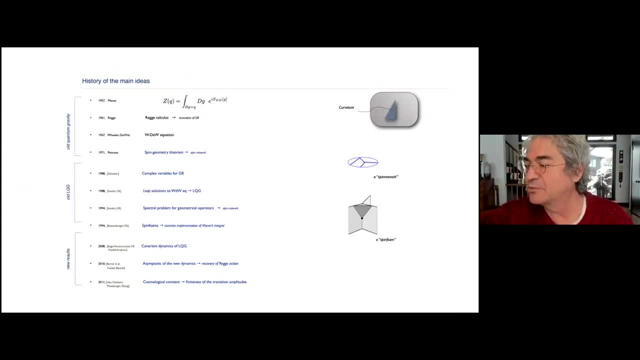 That was most technical And the technical thing I've done, how I'm doing with time I'm pretty well. So I want to close with various comments about what one does with that, how one got there and comparing with the overall picture of the research. 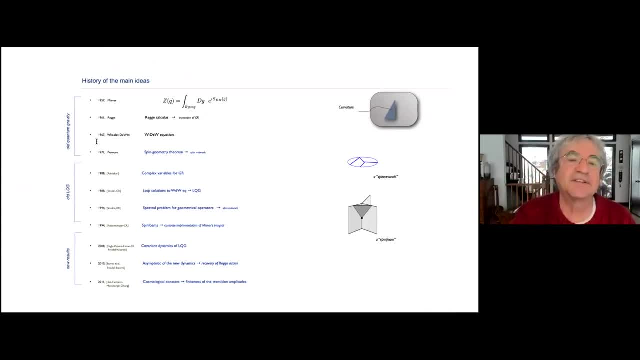 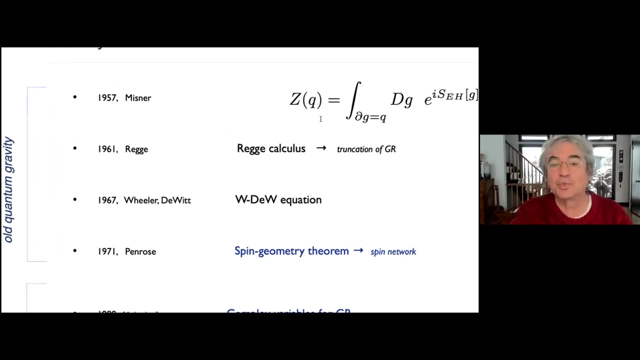 on quantum gravity. This is a slide with a very rapid overview of the history Quantum gravity started. it's very small. I don't know if you see these things. It started back in the 50s with Misner, who's the first one. 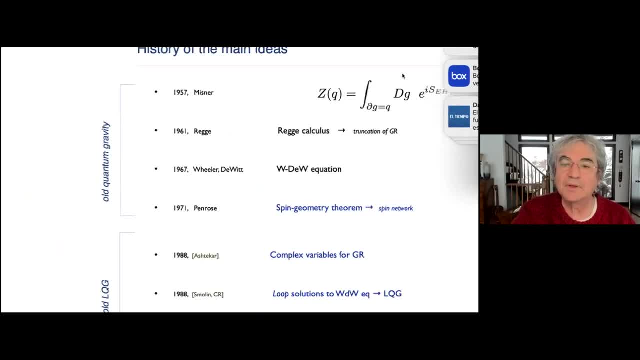 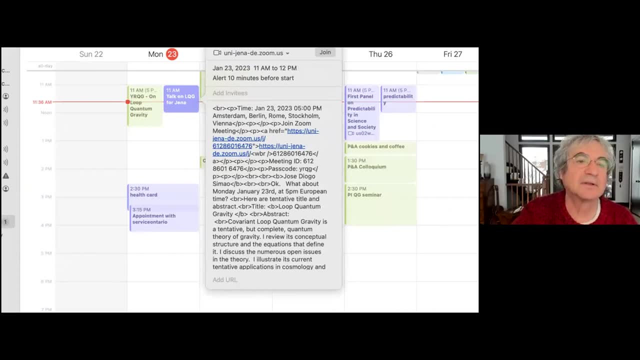 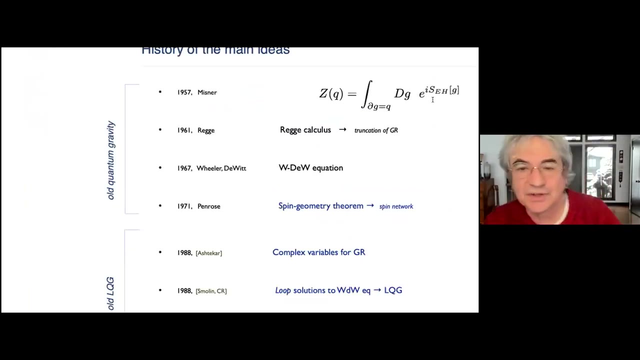 who wrote this? oops, who, oops, sorry coming in the way- who wrote the function into quantum gravity? Essentially, what I've given you with the transition amplitude is a version of the function. It's a function of quantum gravity. 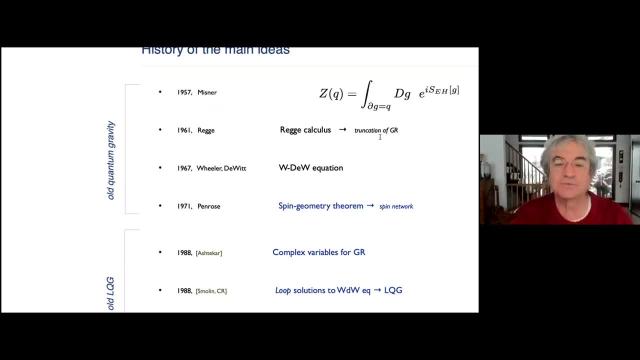 discretized the sort of, but in a way that works better than reg. As you all know, in the 60s there was the basic development of the idea of quantum gravity with Will DeWitt, And in the 70s Penrose came out with this spin geometry theorem. 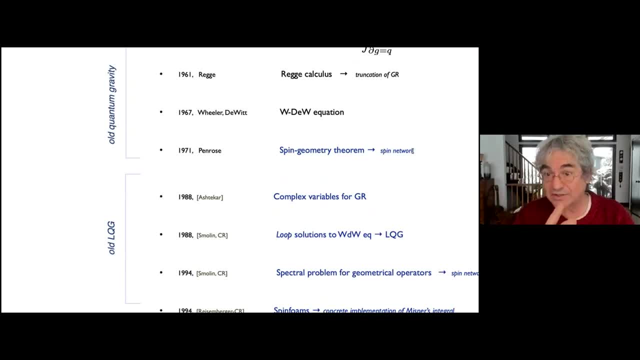 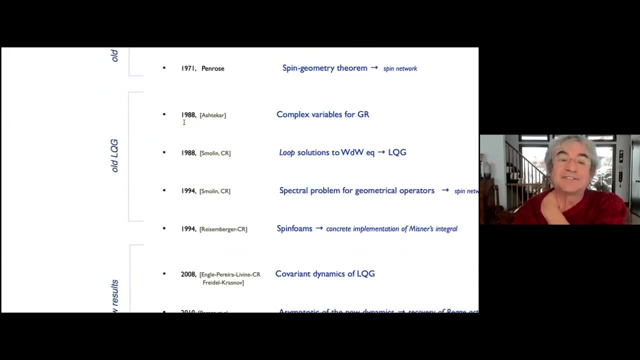 which is the core of the spin network geometry. This is a way of describing geometry: three-dimensional quantum geometry. that I told you. So this is sort of the prehistory. Look, quantum gravity started in the 80s. It's a classical work by with a complex variable. 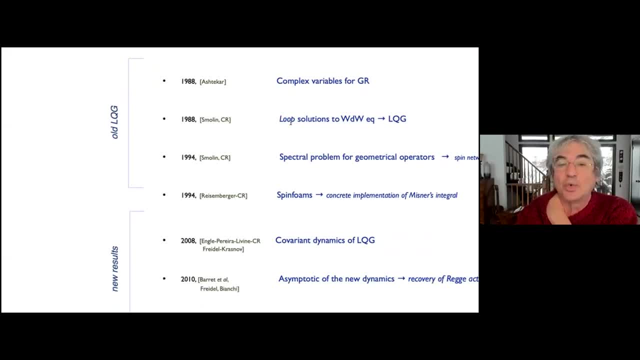 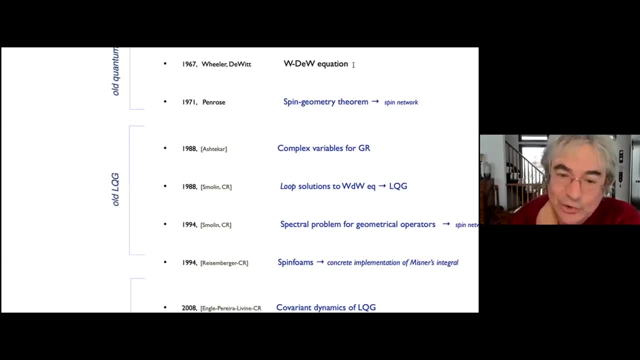 And then, with Smalling, it exploded because it realized that equation has solutions once they are written in the variables, And these solutions are loopy. So the idea is say, OK, good, go to the basis of this solution. see what happened. 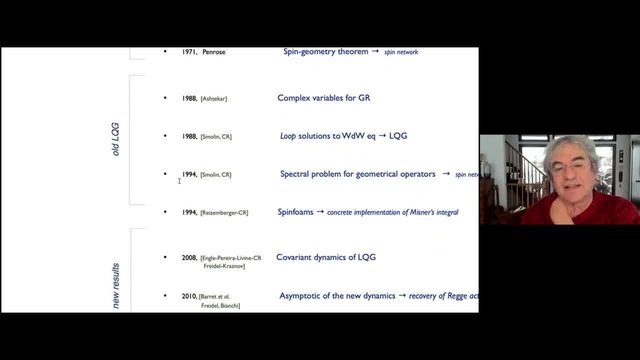 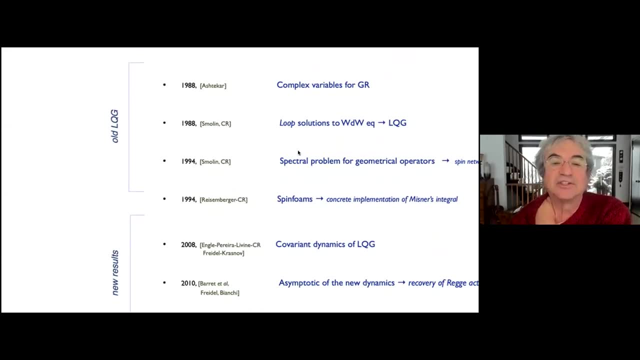 And this was the beginning of loop quantum gravity And the key result of the discretization of the geometry in the middle of it in the 90s were the calculation of the spectral problem And in the 90s also the idea of doing the covariant version. 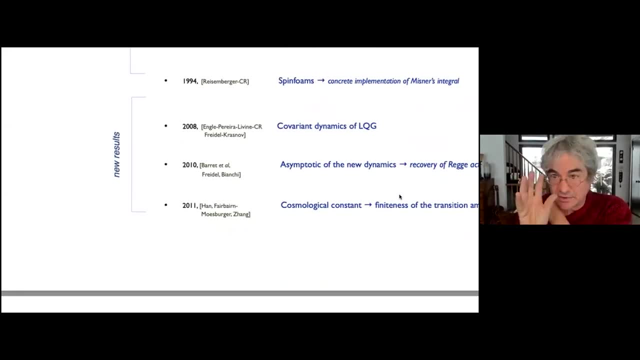 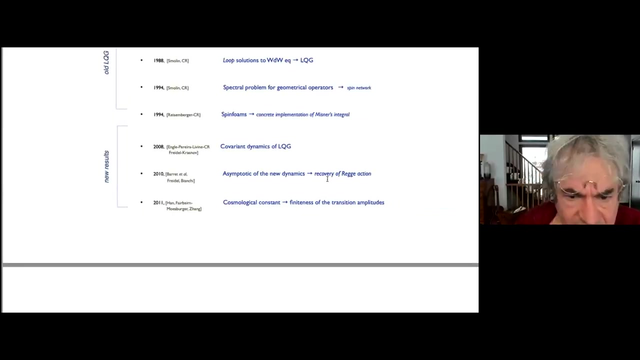 began. The actual expression of the transition amplitudes is 2008,. after a sequence of attempts And shortly after, there was the proof that the limit of this transition amplitudes is, in fact, general relativity. One gets the limit in the end. 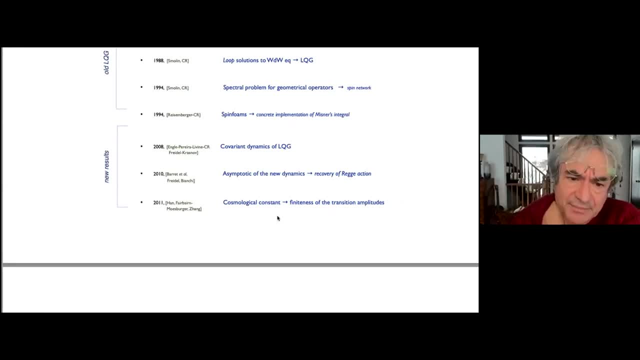 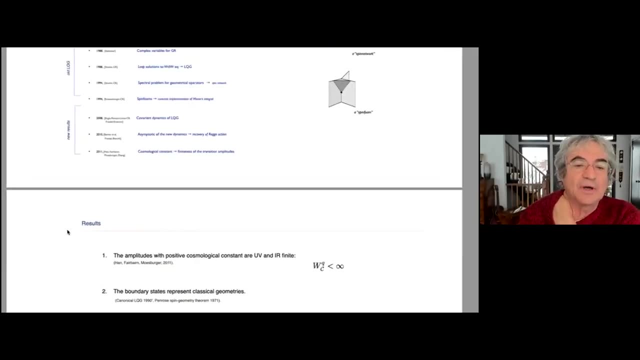 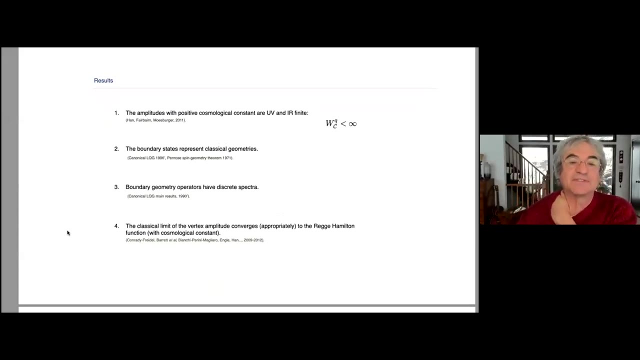 And theorems about finiteness came up shortly later. Now the key results of the theory are these: The amplitudes are finite. The boundary state represents The classical geometry, The boundary geometry of this big spectra, And the classical limit of vertical amplitudes. 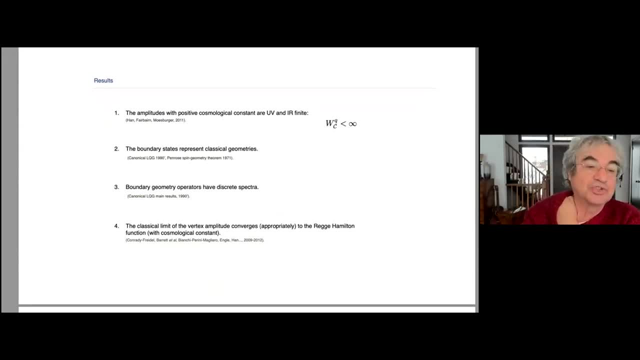 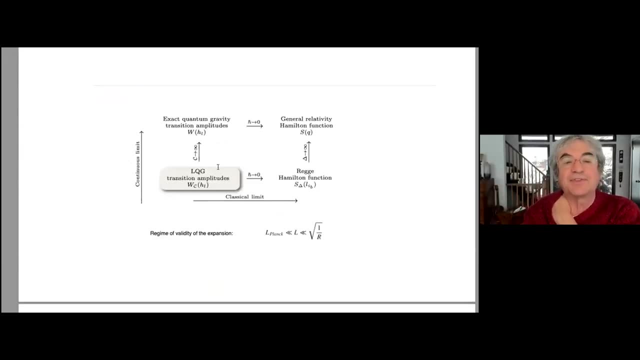 is exactly the range Hamilton function which is in turn such a limited general relativity. So the way of thinking about this is that this truncated amplitudes approximate exact amplitudes which we don't know how to write, And there is a classical limit which gives. 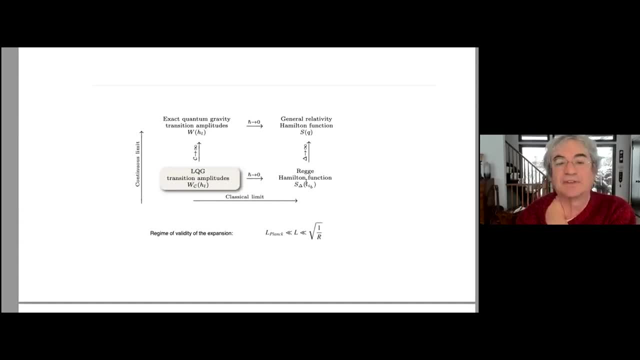 a discrete classical theory And which in turns, in the refined triangulation we know it, gives general relativity. These two limits- actually it has been understood recently- have to be taken together. They cannot be nicely separated in this picture. 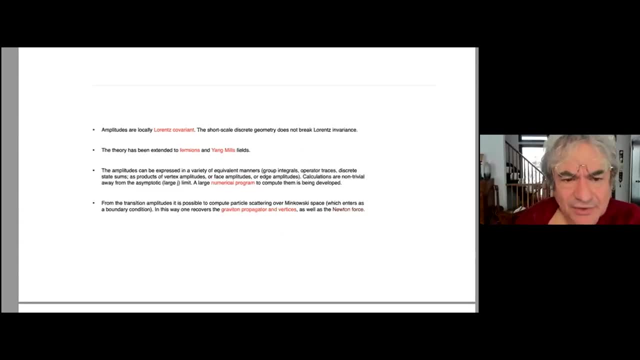 But this gives the idea of how things work. Series Lorentz: covariants can be coupled with fermions and Yang-Niels. The transitional amplitudes are hard to compute, even if they can be written, And they can be written in 10 different ways. 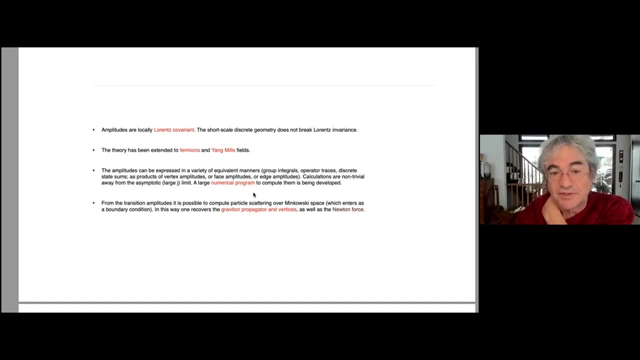 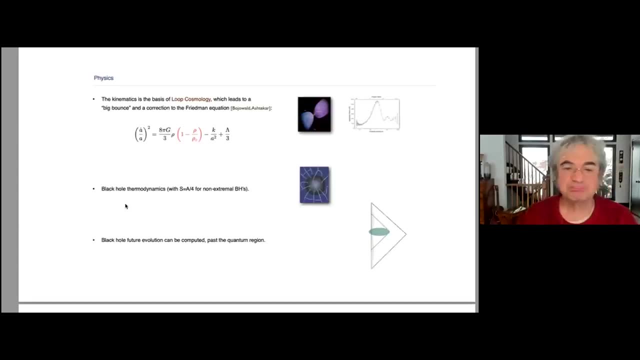 So now there is a beautiful numerical program which has been developed, the codes for computing that and a lot of numerical activity in that direction. OK, so that's the theory. What does one do with this theory? What is the physics? 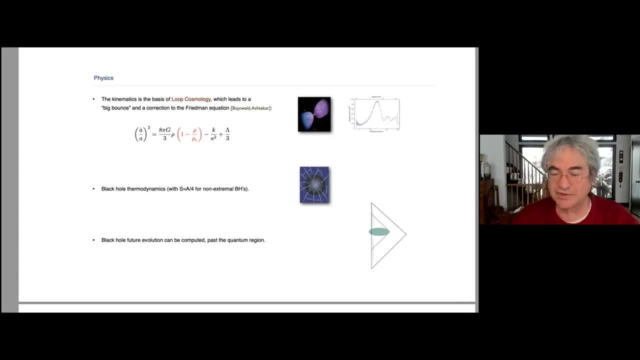 The domain applications are two. One is cosmology. There's a huge field which is called loop quantum cosmology, which is the theory of the, And what you can do is you can take the theory, some of the result of the theory, and approximate dramatically. 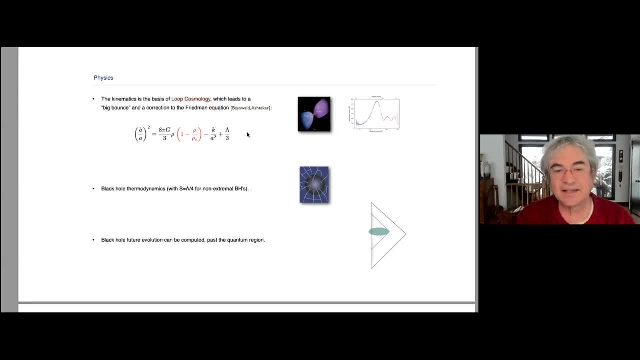 to a cosmological situation and see what happens, And the pretty solid result is that the Friedmann equation gets corrected with a term And this term has a result that if you walk, evolve the state back in time, it bounces instead of the Big Bang. 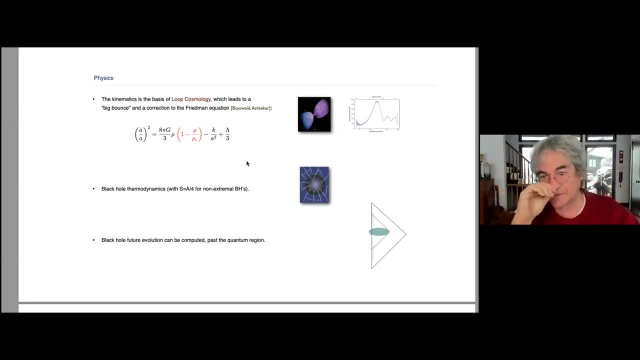 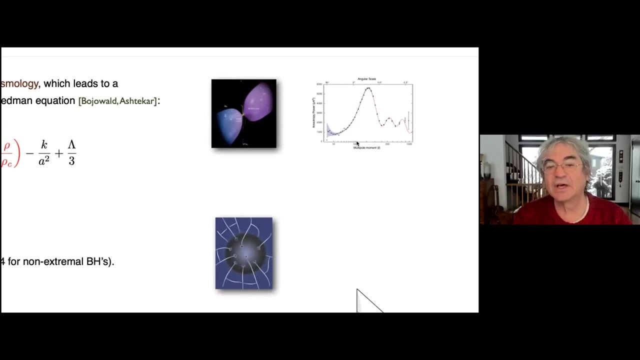 There was a contracting phase and then an expansion And a lot of work. it's sort of expanding around this and using again result from the field theory to try to see if in the CMB one can predict something different from the standard cosmological. 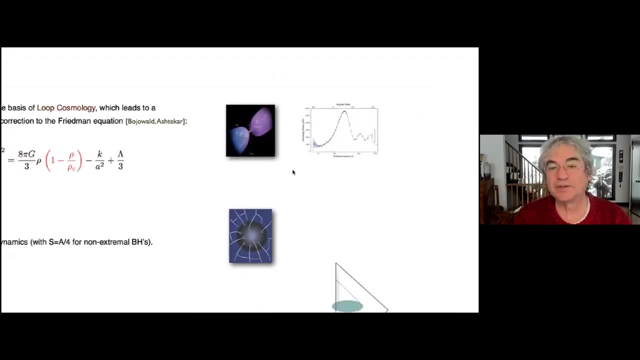 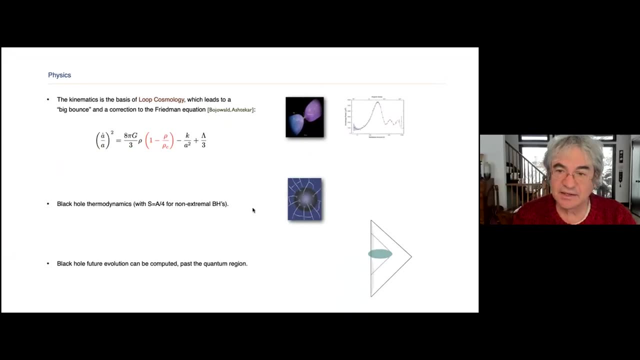 theory, especially in this area. here, of course, and compare with observations, It's a big industry there. A lot of work has been done in black hole thermodynamics, deriving the back-of-the-Oak entropy And the work in which I am focused right now. 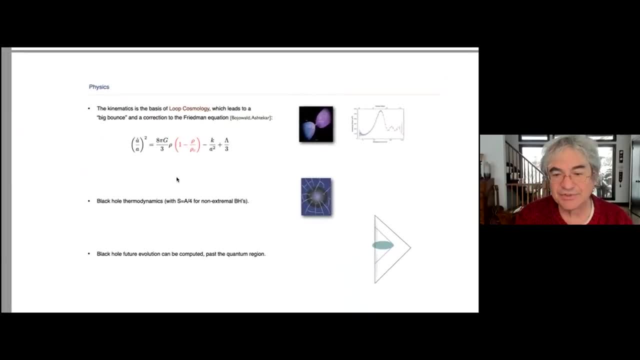 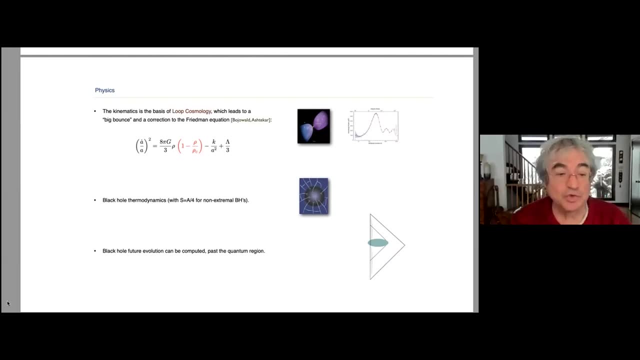 is also on black hole, And this is what I find most interesting going on right now. It's about what happened to all the matter that falls into the black hole and what happens in the future of the black hole. So there is a standard picture that says: 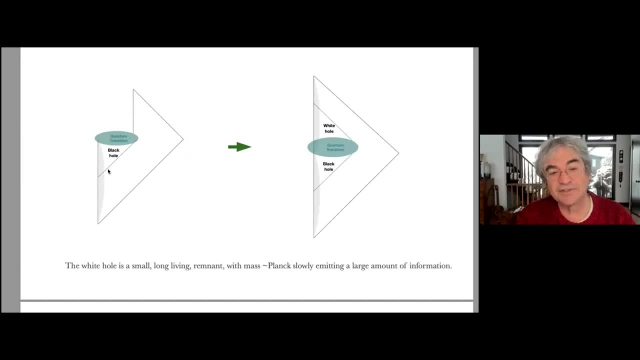 if you have a star that collapses, you have an horizon that form, there is a Hawking radiation, the star evaporates and then it disappears. This picture, I think, is silly, because we have no theory whatsoever that tells us that the thing disappear. 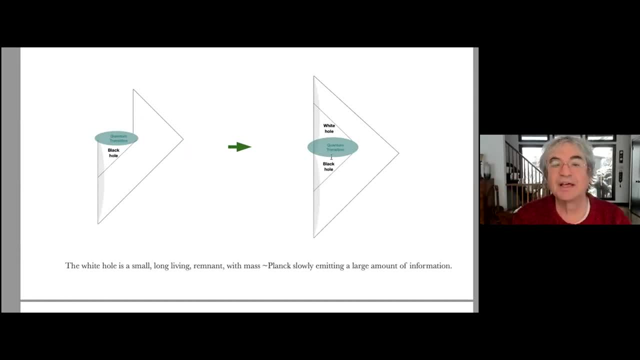 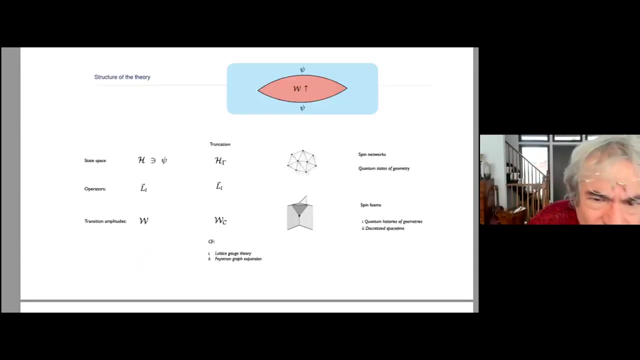 I think that the credible picture is something else. There is a quantum transition amplitudes to something else And if you work through the theory you can see you're exactly in the situation in which you can use the, the covariant logic. 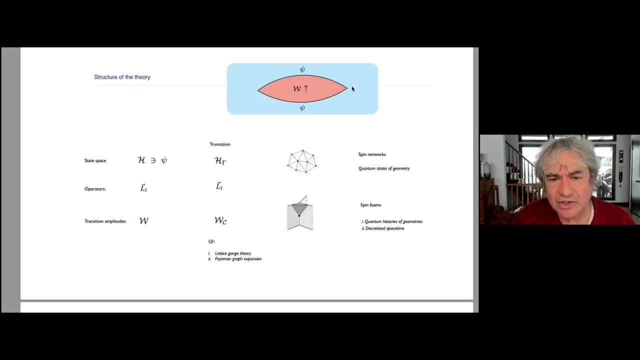 Remember this picture here. This is the logic of the theory. You have an external region where you can forget quantum gravity because the classical presumption is good enough, And then you have a region where there is a quantum gravitational process. That's how we use quantum mechanics all the time, right? 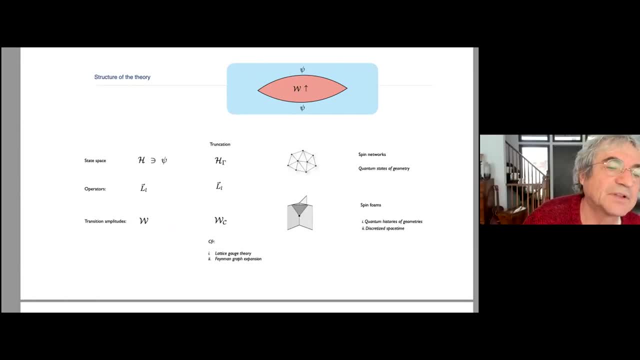 So that's exactly the way to think about black holes, because where it is Here, Because We have a star collapsing, an horizon forming, And then, of course, there is the quantum region, which is the high curvature region. So you just enclose this into a compact domain: space-time. 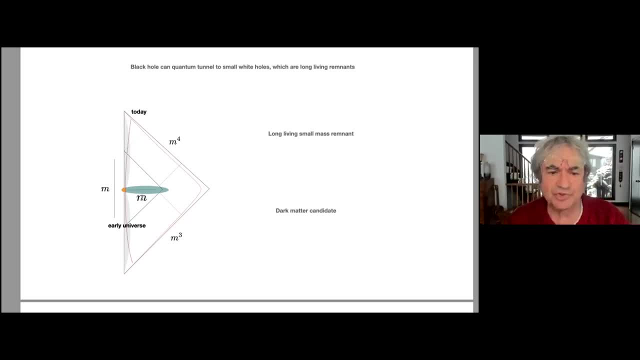 domain Outside the classical approximation is good and you have to compute what happened And this can be done with the transition amplitudes which I gave you. And there's a lot of work. You have to do a lot of analytical, numerically. 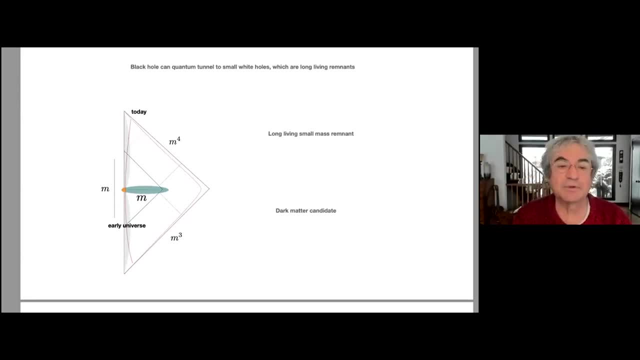 to compute the transition amplitudes, to see what the theory is telling us about the probability transition and so on and so forth. And perhaps one of the things that is in my hope, my secret hope, is that this might be connected to dark matter, because what the theory seems, 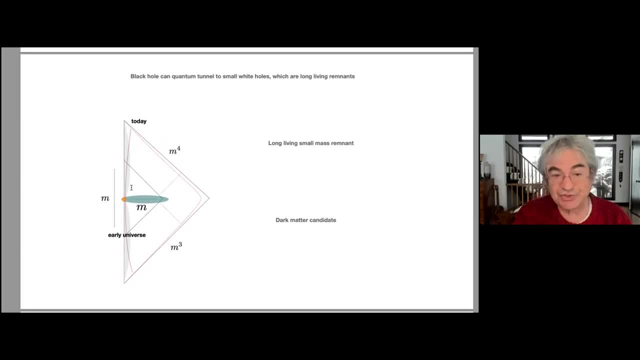 pretty generically to predict is that the interior, through this transition, becomes the trapid region, becomes an anti-trapid region. So a black hole becomes a white hole. So if you're outside, you see a black hole. So if you're outside, you see a white hole. 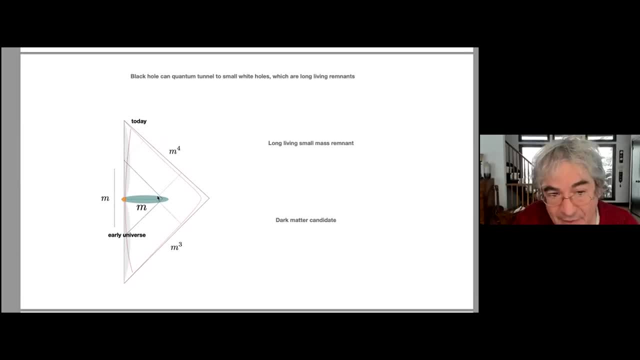 So if you're outside, you see a black hole. So if you're outside, you see a white hole. So if you're outside, you see a black hole becoming a white hole. But of course this happened at the end of evaporation. 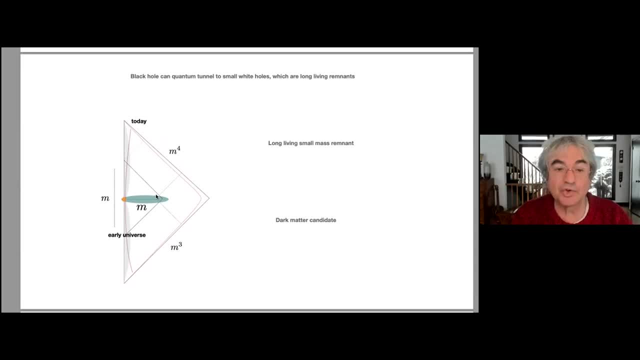 So the black hole has become very small. So you have a very small white hole. that the reason to believe, theoretical reason to believe that it's going to live for a very long time, a time much longer than the Hawking life of the black hole. 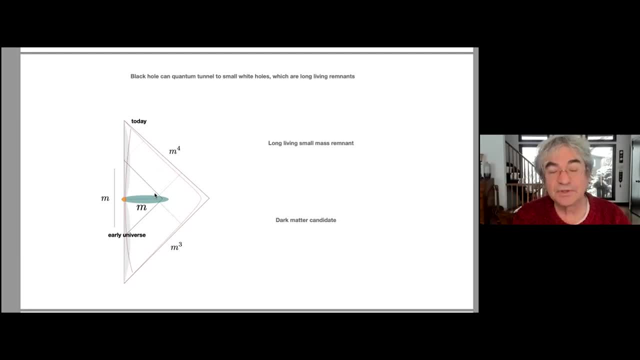 emit very slowly, And so what the theory predicts is that old black holes are all become remnants, those small little things, Planck size microgram, that live for a very long time, which is exactly how dark matter shows itself. So could this be a candidate of dark matter? 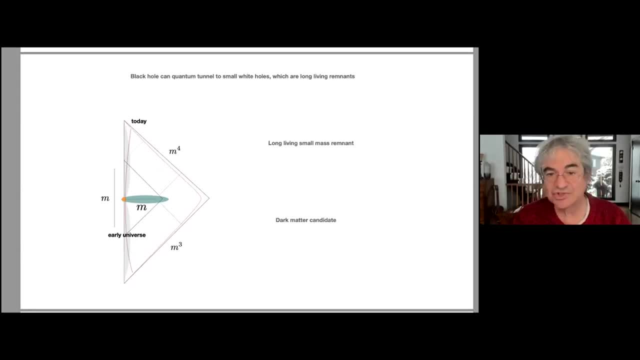 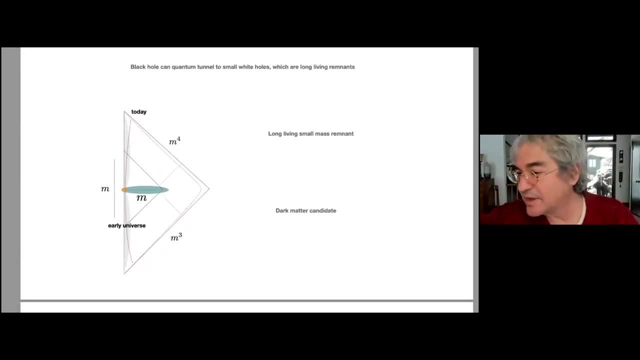 With many candidates of dark matter. that's another possibility. is one challenging hypothesis that comes from the theory Good. So this is all about loop quantum gravity. I've talked for 35, 40 minutes, So I take the last few minutes before taking your questions. 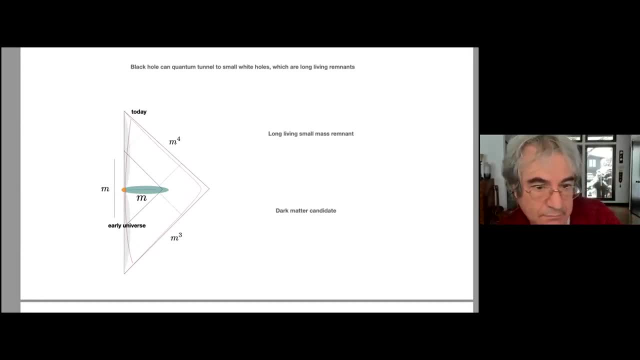 by saying something more general. So I told you about loop quantum gravity: structural theory, characteristic and applications. Now you guys are doing this looking at quantum gravity in general. So loop quantum gravity is just one chapter in the research of quantum gravity. 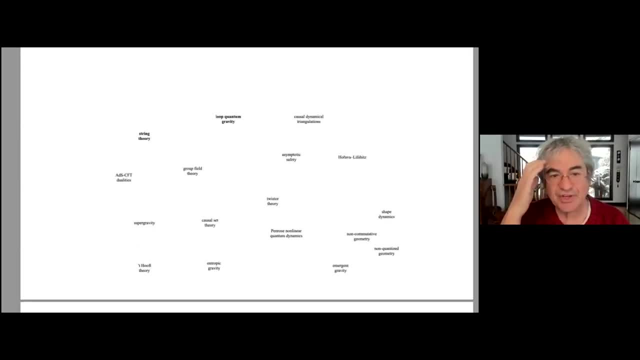 And, as you all know, there are all sorts of approaches. So I'm going to start. So there's a lot of approaches to quantum gravity. This is a scattered list of many of them. It seems daring and it seems there are too many. 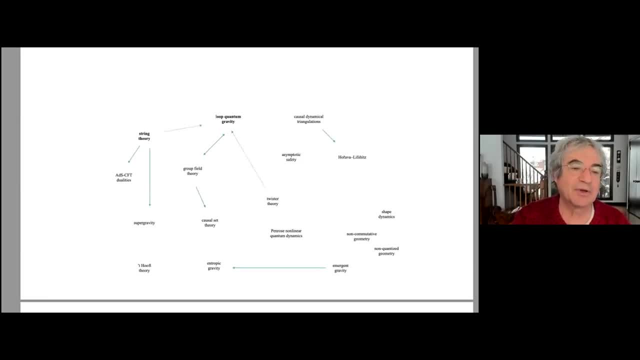 But I think they're less than one thing. First of all, there are connections about that And one can organize the approaches to quantum gravity depending on what are the physical hypotheses which are put into the theory, like violation of Lorentz invariance, like violations of quantum mechanics. 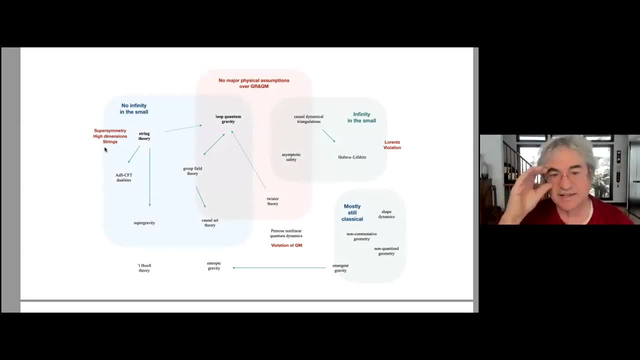 super symmetry, high dimension, extra stuff And perhaps two main areas which I call no infinity in the small and infinity in the small, which are the two major hypotheses about quantum spacetime. This green one is a thing about asymptotic safety. 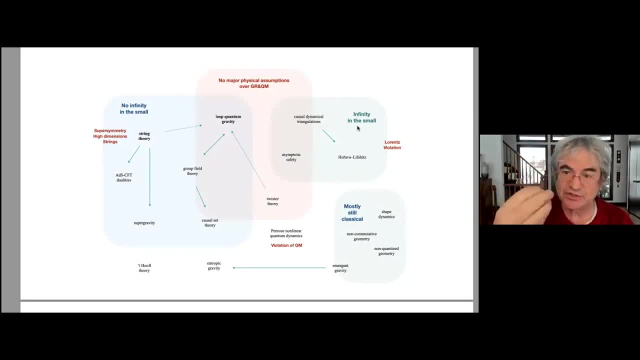 is a hypothesis that there are degrees of freedom all the way to arbitrary small scale or high energy, to infinity, OK. While if you want both, loop, quantum gravity, string theory are characterized by the physical result, not hypothesis, because this both comes from a result, a quantization. 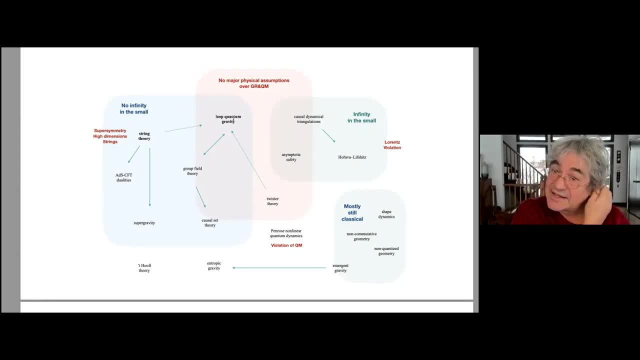 of string or a quantization of the geometry, that in some sense there is no physics beyond the Planck scale. There are no excitations beyond the Planck scale In loop quantum gravity. this is very physical, very direct. It's for the same reason in which a harmonic oscillator 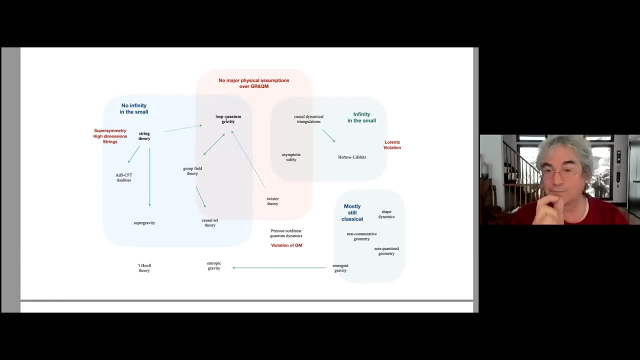 doesn't have oscillations, OK, Less than 1 half h bar omega. the same region of spacetime doesn't have volumes less than something. And string theory: something similar happens right, Because, in a sense, if you want to squeeze a string too much, 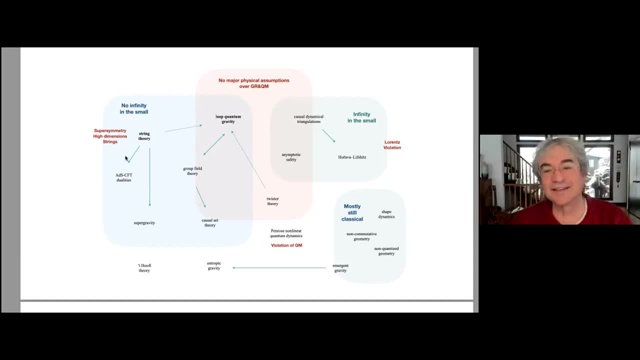 then the other modes of the string get excited. So again, you cannot probe a region smaller than h, bar than the Planck length Or the string length. But so there is some connections and some clear distinction between all the current approaches, But what I want to say is that many of them 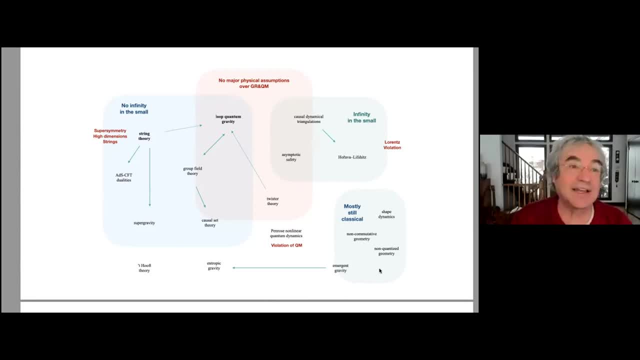 are not really quantum gravity, are just ideas. I mean classical theory, because maybe one day will be useful for quantum gravity. Some of them are very radical, like thinking, thinking that quantum mechanics is wrong And more important. But we do have empirical inputs. 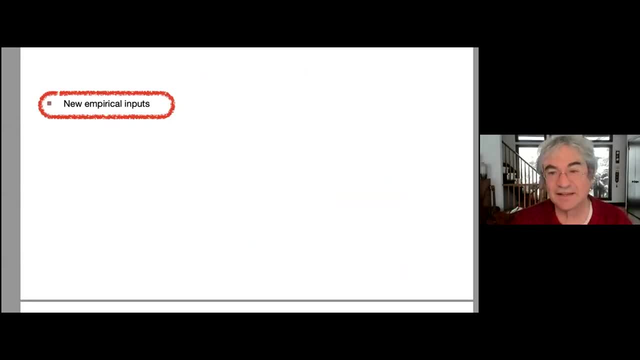 And empirical inputs have come in in the last years or decade, even numerous, and have completely disrupted the situation that was 20 or 30 years ago that we have no empirical input for quantum gravity. Let me mention this, The first one and the most important one. 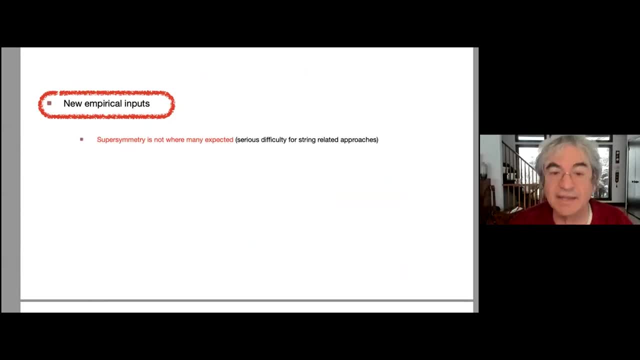 is that supersymmetry is not where many expected. Yeah, And this is a major drawback for string supersymmetry and all related research in quantum gravity. This is not, in the sense of Popper, a falsification of string theory at all. 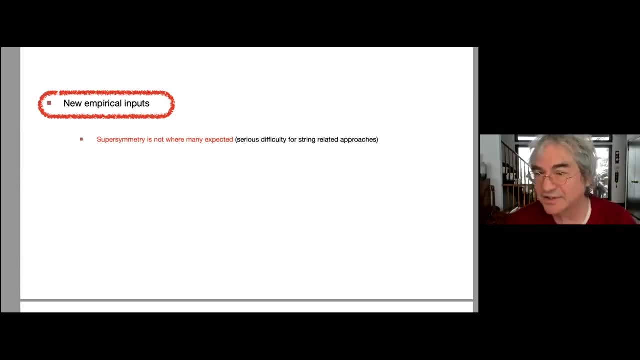 Because of course we know from philosophy of science, you can always take a theory and adjust it to the result, But rarely we have a falsification. The way research works is that some ideas- I don't know They- become productive and tell us something. 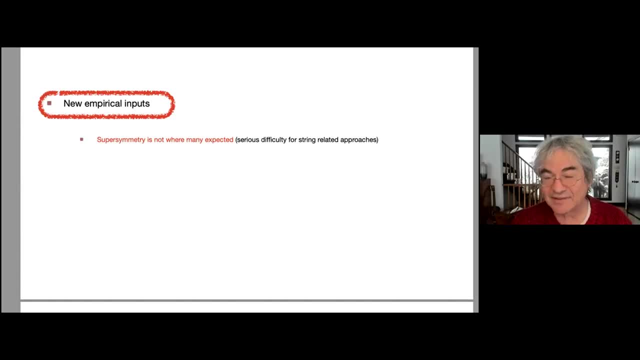 And when an entire community is convinced that something should happen and it doesn't happen, I think it's a strong indication- And people have been talking about the crisis of physics- that the underlying ideas were wrong or not right, not completely right. 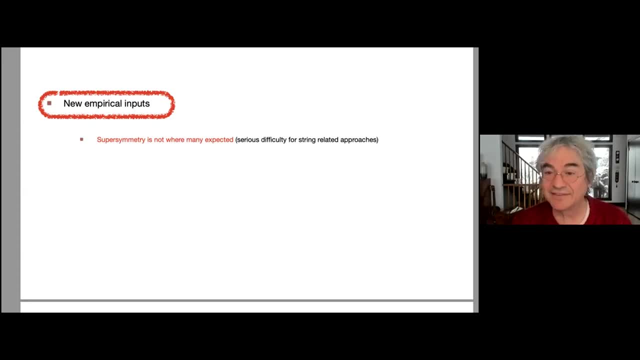 But of course I remember articles, even in France in Le Monde: the crisis of physics. This is not a crisis of physics. This is a crisis of that particular research director that expected supersymmetry. People in quantum gravity did not expect supersymmetry. since decades and thought that no, there's no reason for there's no strong reason. Supersymmetry is a super interesting hypothesis, but it's not so compelling. after all, Naturalness works sometimes, but not always, and so on, and so 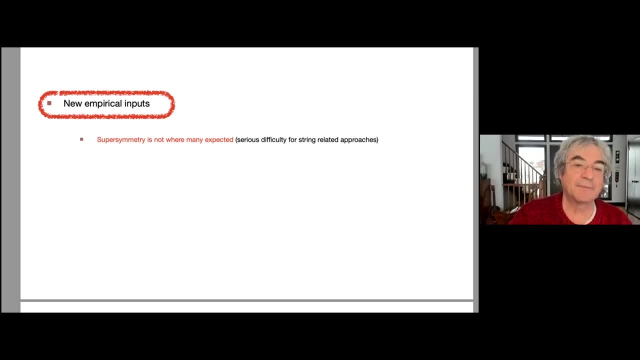 forth. So this is a difficulty for some approaches. Another Difficulty which I think is not emphasized enough, is that same community expected the cosmological concept to be negative, So much that when the cosmologists found it, measured it positive. many theoreticians 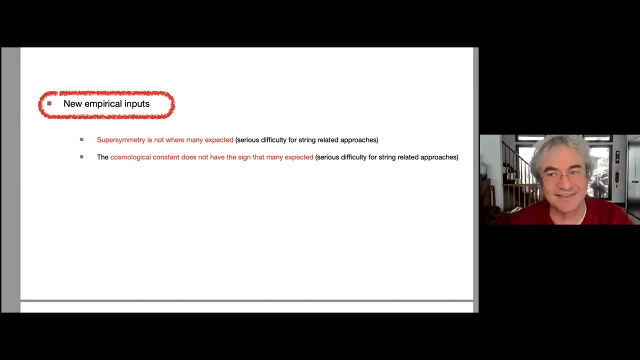 didn't believe the cosmology. It took a Nobel Prize for convincing that they were right, And so much that today a huge amount of papers are published under the hypothesis that the cosmological concept is negative. Every time you read ADS in a paper, it's you know. 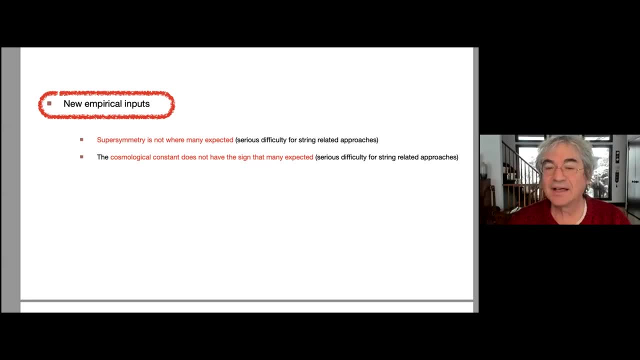 it's an assumption that the world is not what it is With the idea. oh well, but maybe tomorrow we'll find it. we'll find it better. But the cosmological constant is positive. Look, quantum gravity can be written with a positive cosmological constant. 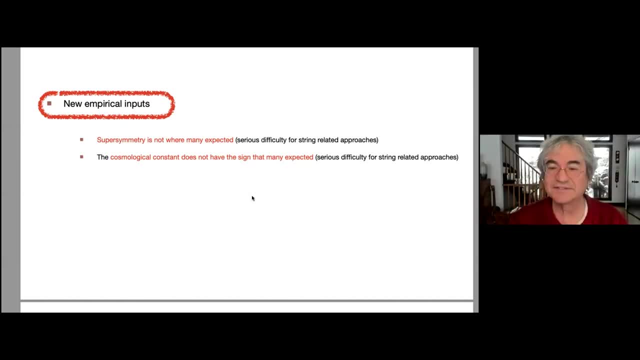 No problem about that. In fact it cuts away the infrared divergences. It plays a big role in the theory And again I think that we should listen to nature, not to physical gravity. Yeah, Other Big empirical inputs that come in. 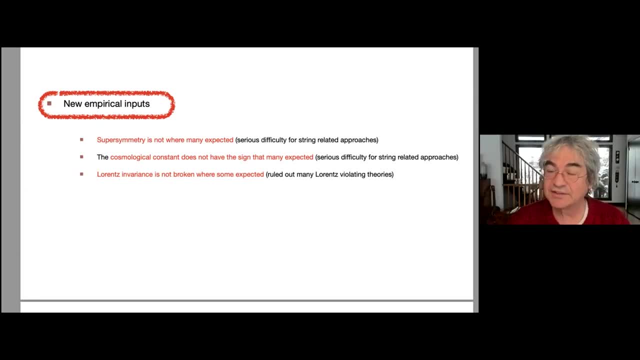 is that this come from astrophysics. There have been a full campaign of research in astrophysics to measure violations of Lorentz invariance because there were papers and papers and papers about Lorentz violating quantum gravity. You can get fine at this by Lorentz violating right. 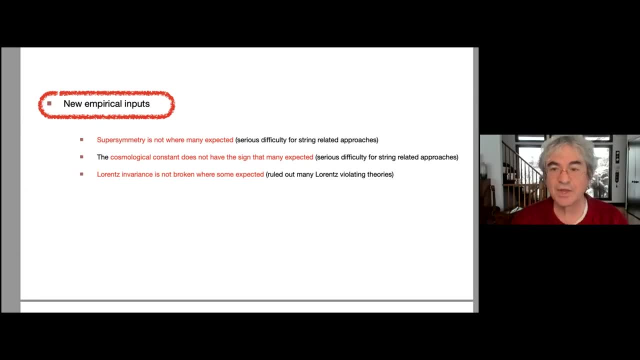 Horschava theory and connection. Well, where the Lorentz violation was expected, it hasn't come out pretty strongly. Now there are big, big, big limits. So once again, these are all empirical results that put difficulties on research directions. 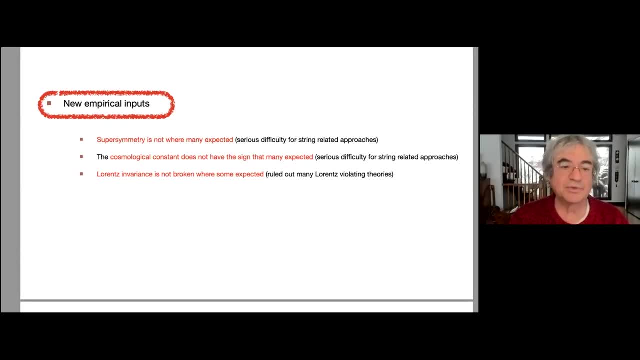 And I think if we are scientists, we should listen to nature, not to our fancies. And recently, another huge empirical input from nature has been the merging of the neutron star, And this is the first time that we've seen a neutron star. 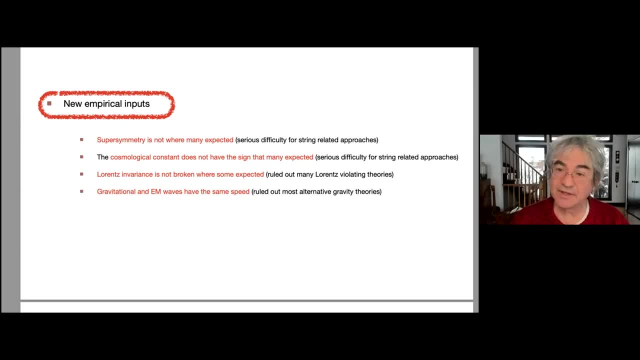 that has been detected simultaneously by LIGO and by electromagnetic detectors in very many ranges of the electromagnetic spectrum. The two signals arrived virtually at the same time, which means that the gravitational waves and electromagnetic waves go at the same speed, which cuts away. This is really a falsification of a huge amount of literature. 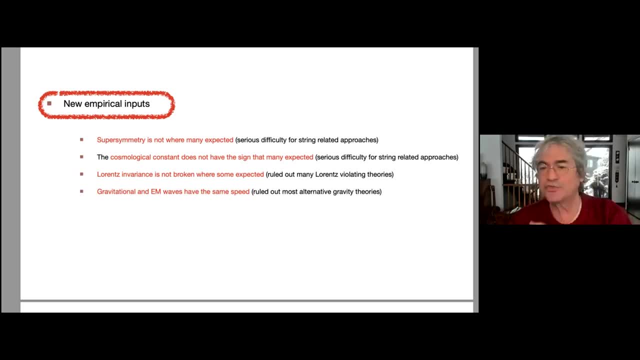 that was exploring alternative general relativity. where this does not work, It doesn't happen. So a lot of FFR, variation of GR theories which were studied by people spending their life studying them. just they're not right. OK, Still, some alternative general relativity is compatible with that. 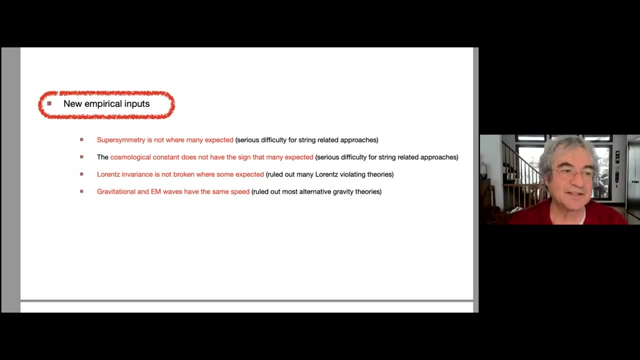 But when you develop a research program that strongly indicates something and it doesn't happen, I think it's that good science says: just look somewhere else. Now I'm not saying, of course, that there are positive indication for loop quantum gravity out there. 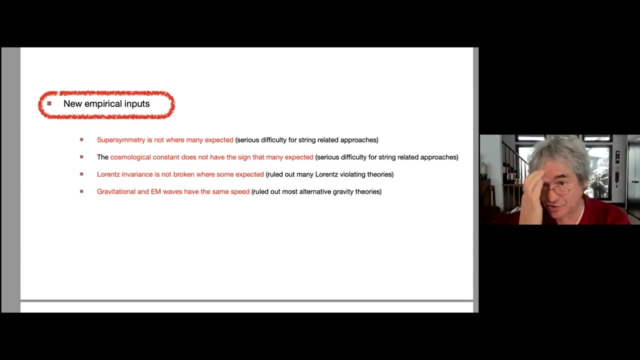 There isn't any- OK, There isn't any positive indication for any approach to quantum gravity, But none of this affects loop quantum gravity in any way. So in a sense, I think loop quantum gravity is a much better situation empirically, not because it will go directly, but because it will go. 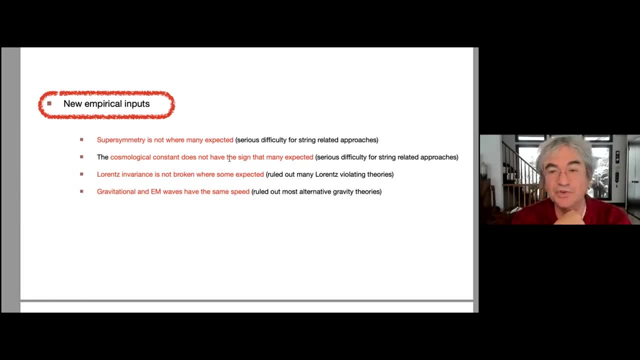 directly to support because the strongest competitors are much in trouble. in the last years- And I also want to mention something which has not been measured but there is a hope to measure in the future, a few years, nobody knows- which is the quantum superposition of geometries. 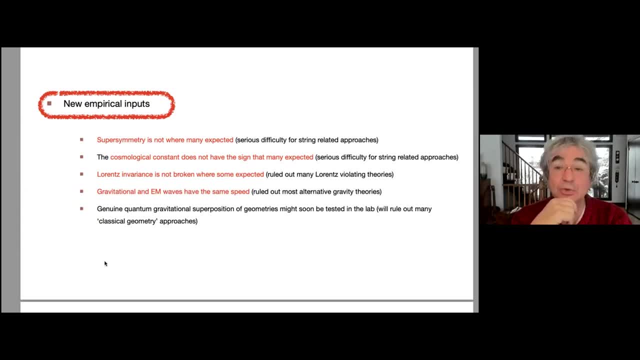 to be measured in the laboratory in a non-relativistic case. This is a spectacular development in the last, in the last years. It's a sort of a regime that nobody paid attention much. There is a non-relativistic regime, quantum field, theoretical. 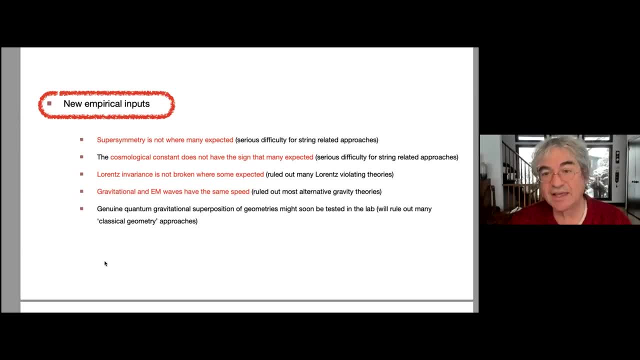 in which you can put instant superposition, quantum fields and measure system getting entangled through that, which would rule out if it is measured and many people would bet that the result would come out from the experiment. would rule out all the speculations. 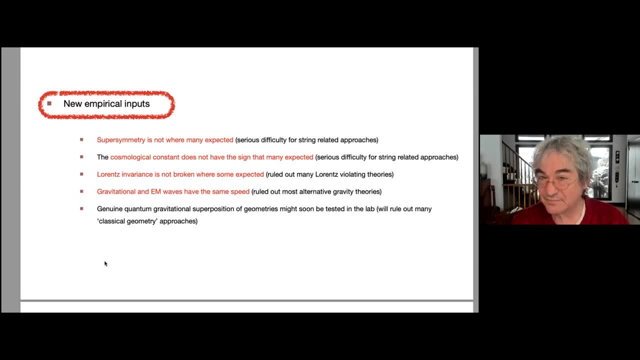 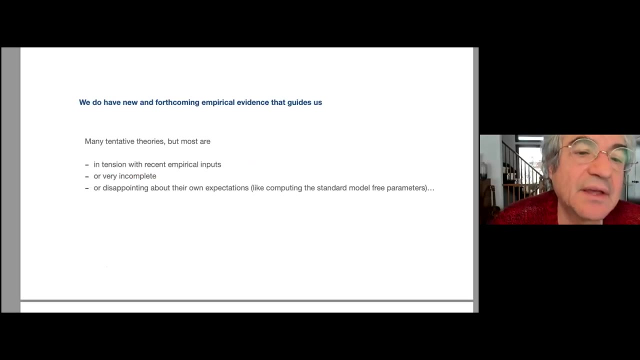 about gravity being classical, Because this is an effect which is not predicted by all the theory I know in which gravity is classical. Good, So we have many directions for quantum gravity, but many are intentional. with recent inputs, Many are extremely incomplete And our theories are just half-cooked idea. maybe from this: 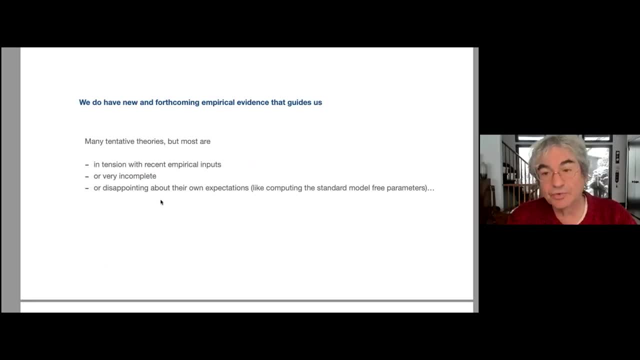 will go somewhere. Yeah, Yeah, Yeah, Yeah, Yeah. Many- and I also want to mention this separately- have been very disappointing on their own expectation. Remember that when I was your age, guys, string theorists- were sure that they would be able to compute all the standard model. 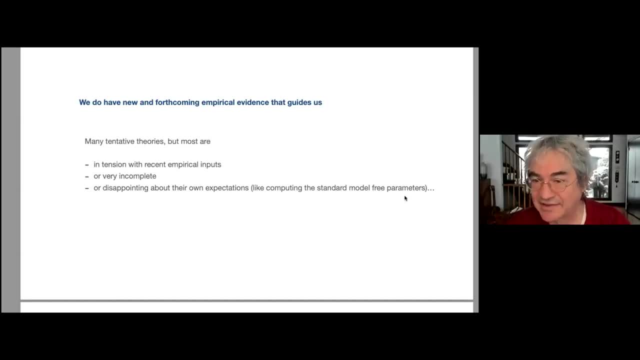 free parameters in a few years. 40 years have passed and nothing has happened whatsoever. So the number of theories. but there are well-defined quantum theory of gravities unproven. And they are not the only theory, but there are also some other theories. 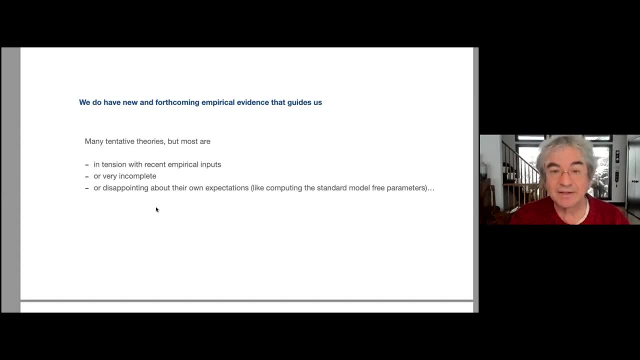 that have not been proven to be true, And I think these are the theories that are very important to be developed: not yet clear but definitely complete quantum theory of gravity, which might be right like quantum gravity. I close with what I like about all this as a theoretician. 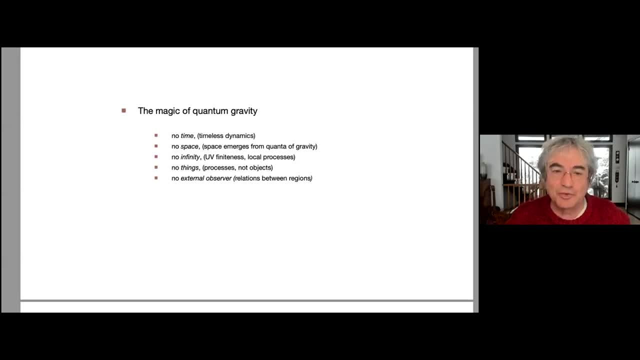 If you look at the theory, the stage it is now, I think it's beautiful. I think it's beautiful, but I don't know what it's going to be when I start and went into the field. The theory is formulated. if you think of the equations that I gave you, 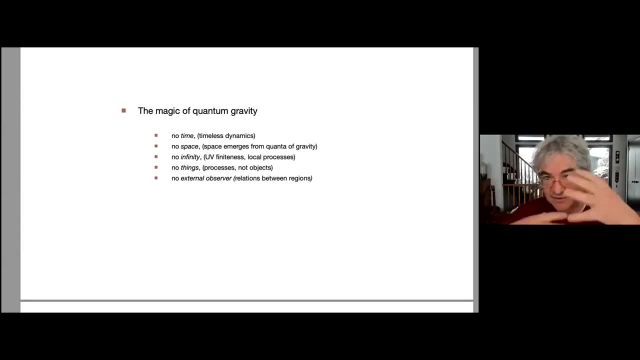 there's no time variable, So it's a fully time-lapsed dynamics. in the sense it's a relational dynamic. Describe very well the world in which we are without an external time parameter. Space is not a variable. There are no coordinates in the theories. 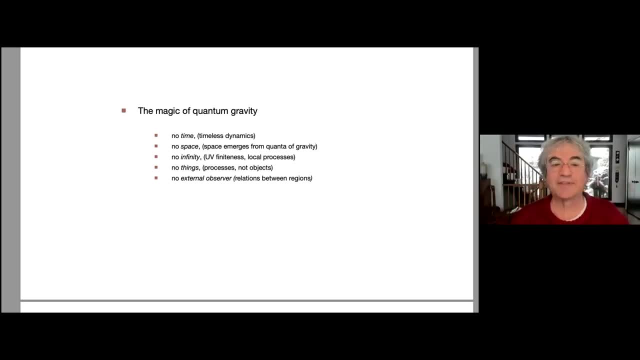 What we call space emerged by the quanta of gravity attached to one another. Space, time, matter, everything, geometry, it's all quantum fields. It's not a unified theory in the sense that there is a single thing that becomes fermions, Young-Mills and gravitational fields and so on. 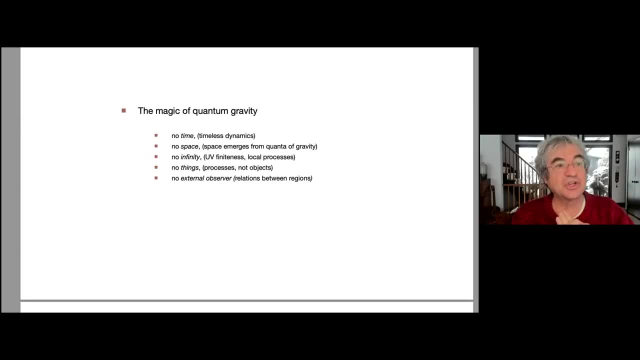 but it's a conceptually unified thing in which there is a single set of entities which are quantum fields, general quantum field theory, which gave rise to fermions, Young-Mills, gravity, space and time. There are no infinities in both sense. 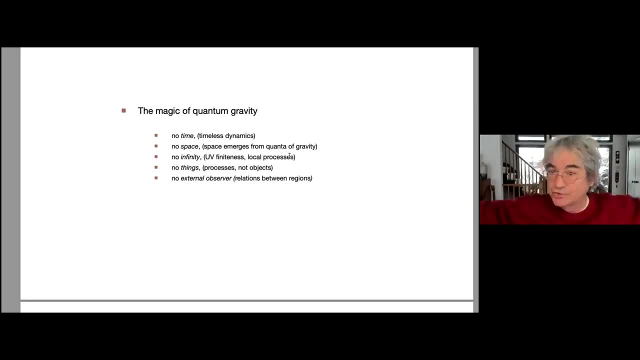 It's ultraviolet. but also you don't need to go to a synthetic infinity. You can do everything in local processes And there are no things in the sense that what the theory is about, if you think about it, but because you describe evolution. 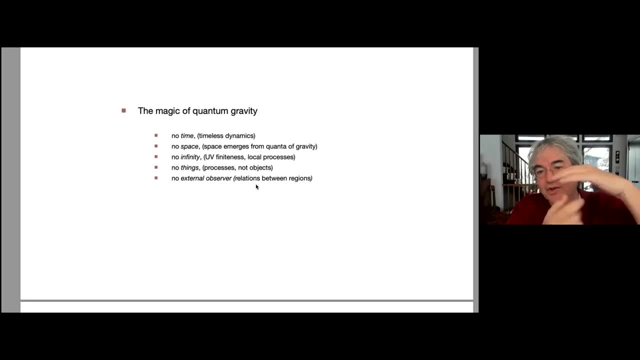 you decide processes, There's no priori way of identifying the same thing across the process. So the theory is about processes, not about things, And there are no external observers, in the sense that if you think about quantum gravity this way, you are not allowed to think. 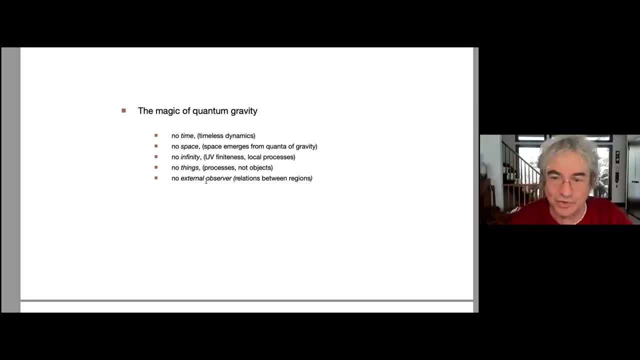 about the observer outside the universe. There's no wave function of the universe here at all. There is pieces of space-time seen from the outside, and so there is how one part of the universe observes another part of the universe. All this I find the beauty. conceptual structure of quantum gravity. 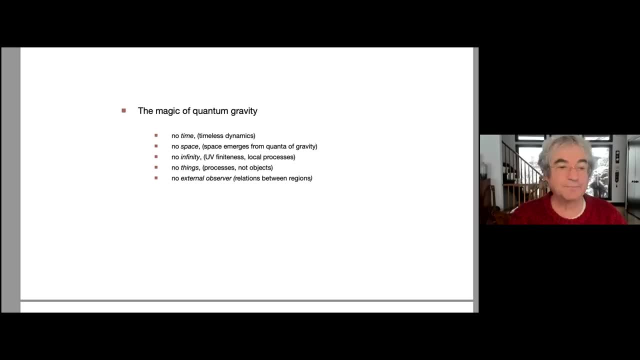 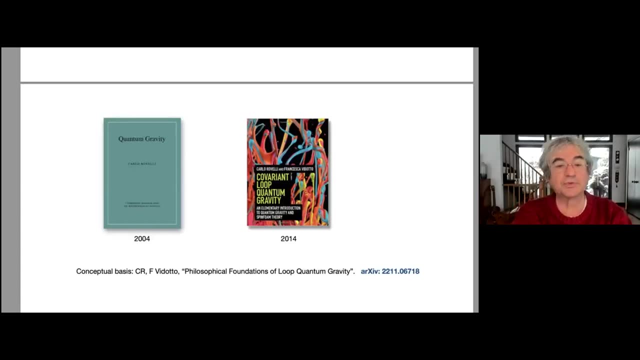 in the ways used in loop quantum gravity. So my last slide is just my two books on this. If you want to go into that, I have an old 2004 book. It's called Quantum Gravity. It's about loop quantum gravity, which is more detailed, conceptual. 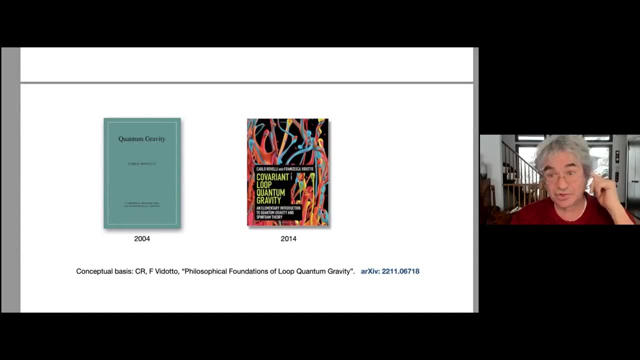 all the stories and a more recent work where there is the transition amplitudes that I told you, much more interactive, much more straightforward, much more simple. So, on the conceptual points, how to do a theory without time, and so on,